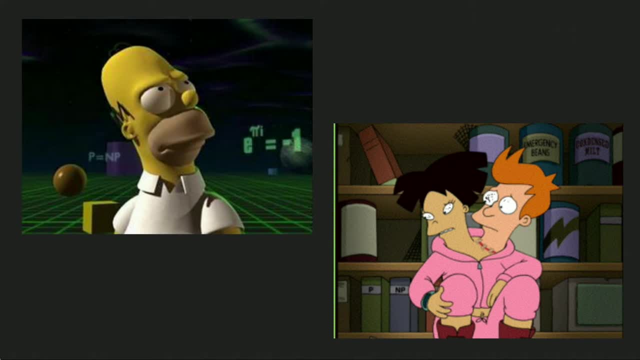 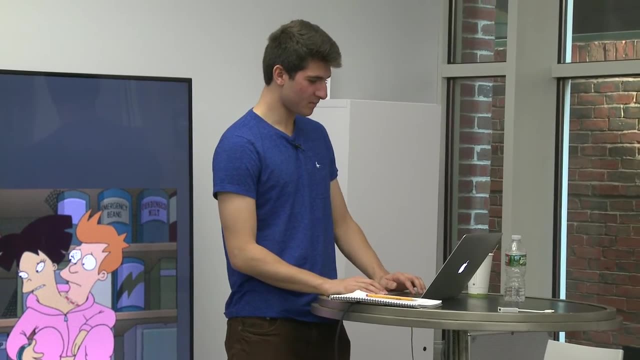 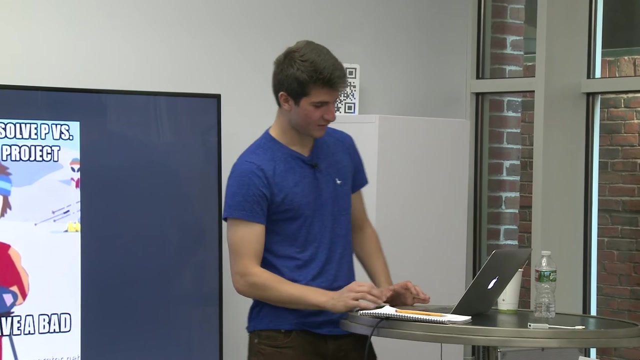 also a Matt Groening production- P and NP in separate books, sort of implying that P is not equal to NP. So that's you know. really, the question is whether or not P is equal to NP, and we'll get into what that means in just a second. But if you're watching this and you're thinking, 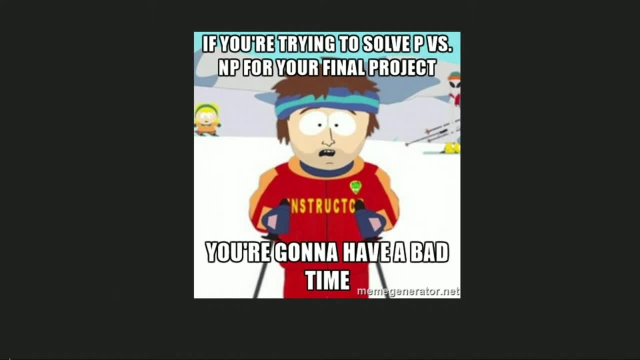 hey, I want to solve P versus NP, for my final project got some bad news. It's probably not the best idea. Don't want to discourage you, but a lot of really, really famous smart people- much smarter than me- have tried to solve this problem for a long time And I 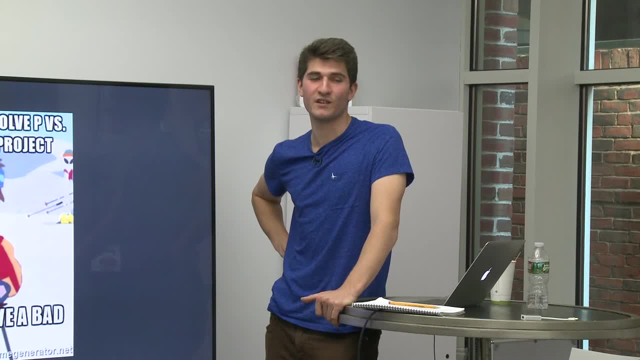 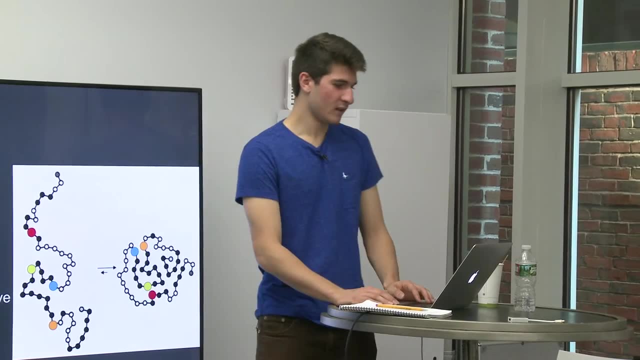 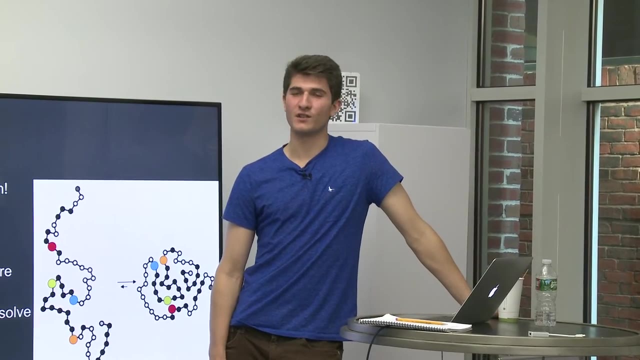 think we can learn a lot from it, but the problem may not be solved for a long time. And yeah, I mean, why should we care about the theory of computer science? In CS50, you learn a lot about the running time of algorithms And we talk a lot about how algorithms work. 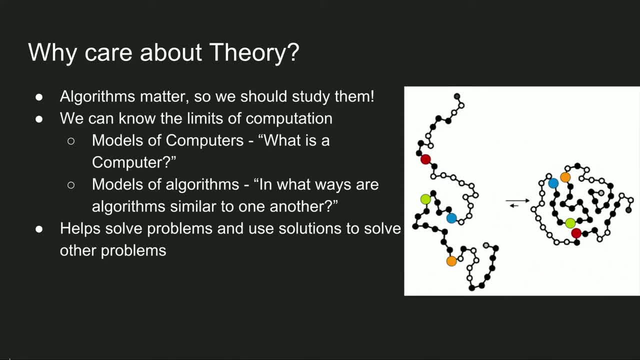 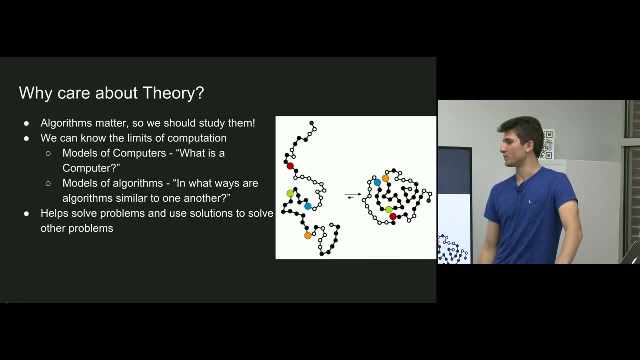 and like what are the best ways to solve certain problems? But theory of computer science sort of goes into like how can we extrapolate from there and what are the sort of fundamental things about algorithms that make them similar to one another and different from one another? 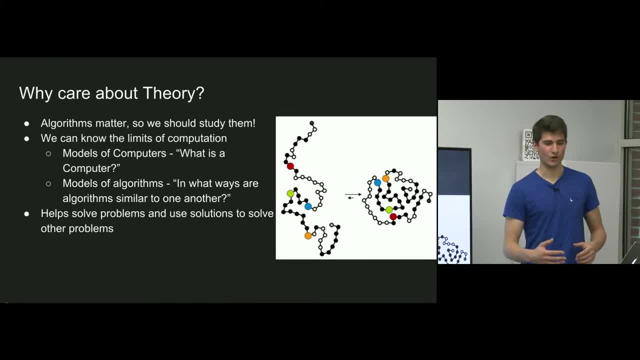 as well as how to model a computer in its simplest form. That's something that Alan Turing did way back when and he sort of became famous for that. I mean, not everyone, but a lot of people are familiar with Turing machines. That's sort of his theoretical model of a. 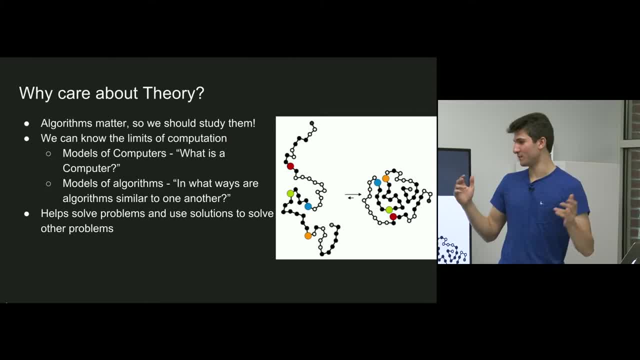 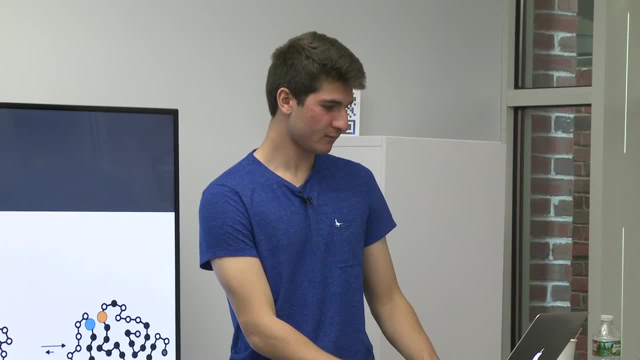 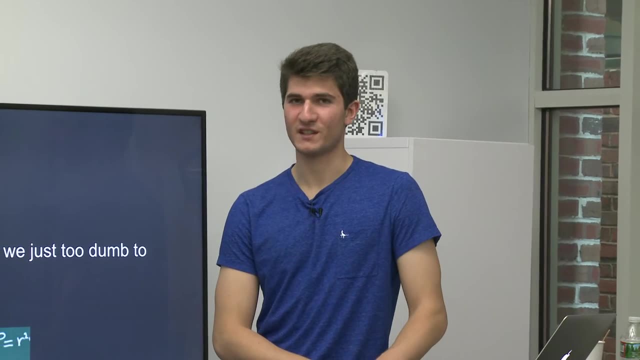 computer And yeah, I mean it helps us solve problems and use solutions from one problem to solve other problems. So it's pretty profound And yeah, so a little more motivation. Answering this question of P versus NP: again, I still haven't really told you what it is, but solving 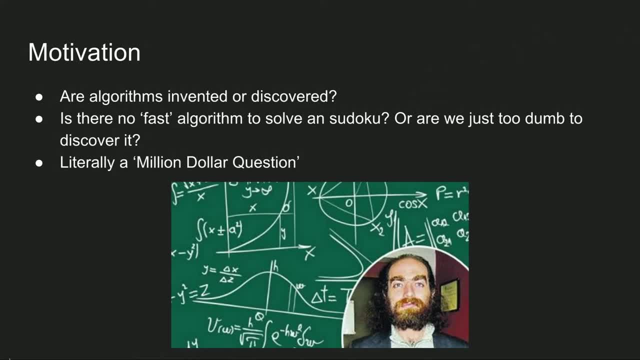 this problem would essentially help us with questions like: are algorithms invented or discovered? Is there some fast algorithm for solving Sudoku that we just haven't discovered yet? Does it just exist in the ether and we haven't discovered yet? Or are we just too dumb to? 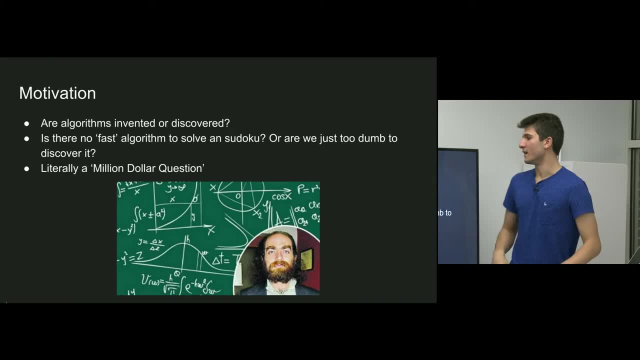 discover it, but it definitely exists, Or does it just not exist at all? And yeah, this question is, if that wasn't motivation enough, it's a million dollar question in the sense that the Clay Institute, it's one of Clay Institute's Millennium Prize problems. 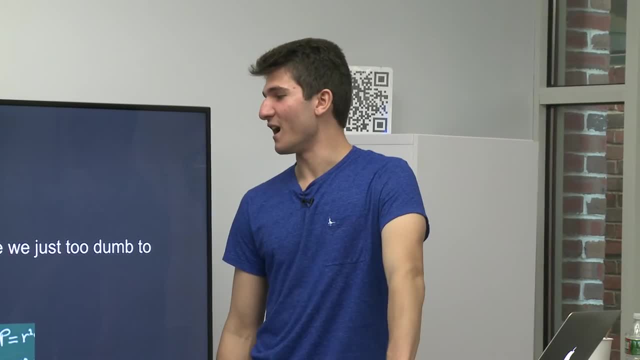 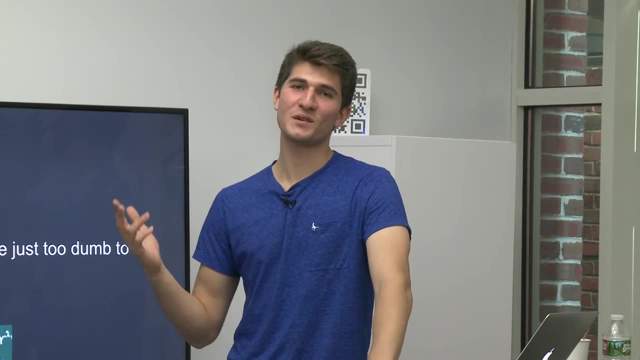 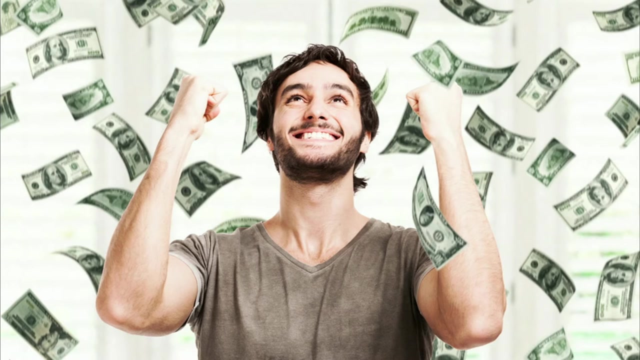 which means there is a million dollars for whoever person can solve it and prove it one way or the other. Because I mean, what do computer science do? What do computer science do Scientists love more than computers? Yeah, money, And I'm hoping that a CS50 student 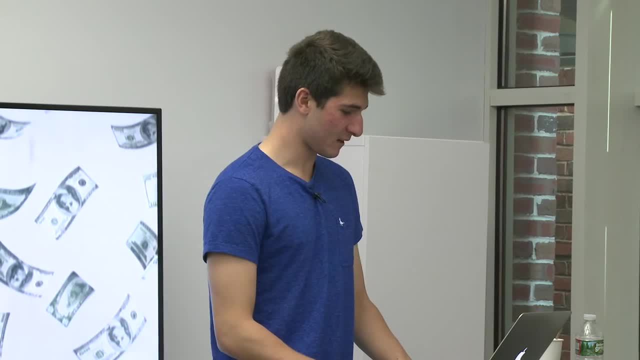 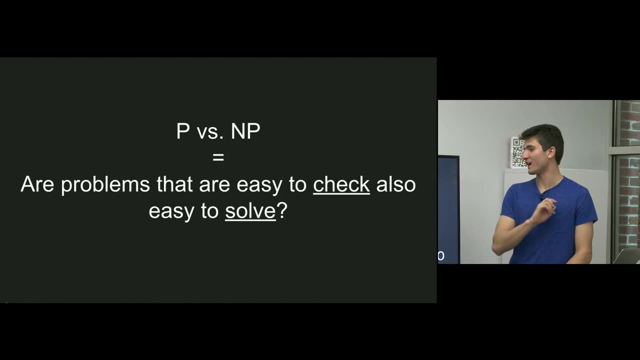 will be the one to solve this problem one day, So I hope you can. So what is the question of P versus NP? And it's really are problems that are easy to check, also easy to solve, And that's sort of a very, very, very very. 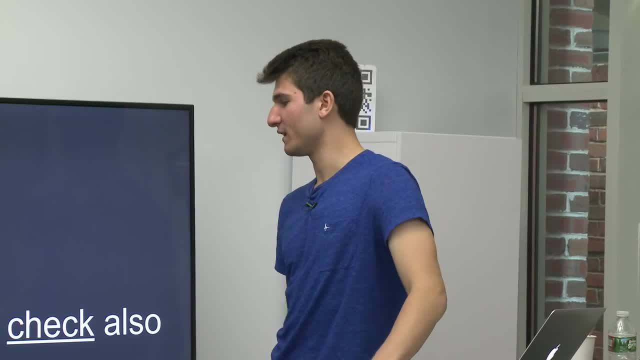 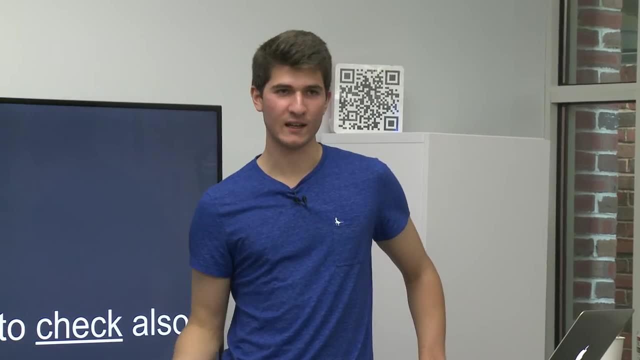 high level thought way to think about it. But what does this word easy mean in this context? What is it? What does it mean to check a problem? what does it mean to solve a problem? hoping to go all of that into all of that in just a minute and hopefully that. 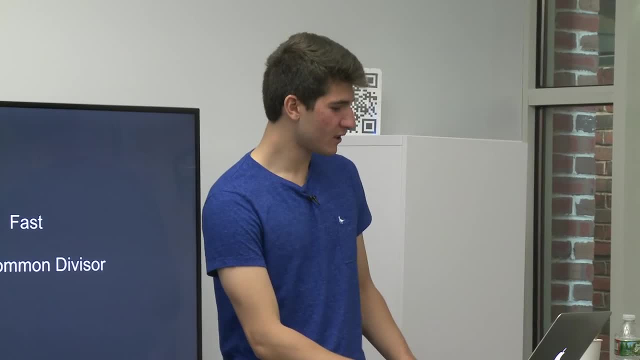 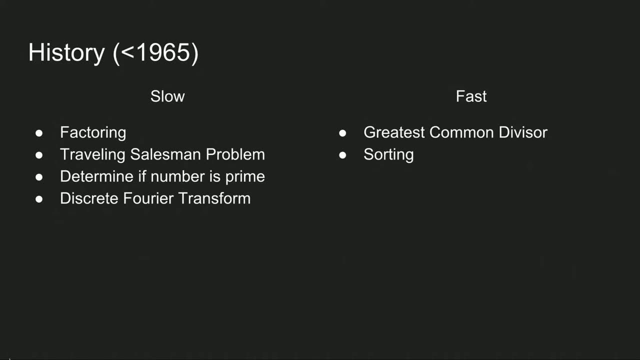 will become clear. So, yeah, this, this problem in particular, has a long history. Back in the mid 1960s, when computers are still the size of cabinets and small houses, people were still trying to find algorithms to solve, you know, basically all the world's problems like factoring and 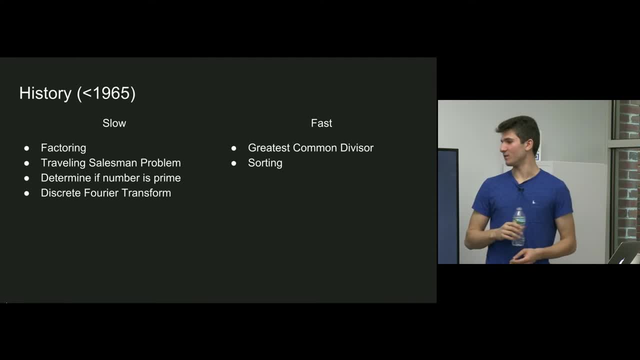 the travelling salesmen In problem, and determining if numbers prime Go All of a sudden got it pluged up And P versus NP in 2016 was one of the problems that US sellers had when and determining if number is prime and problems like these. 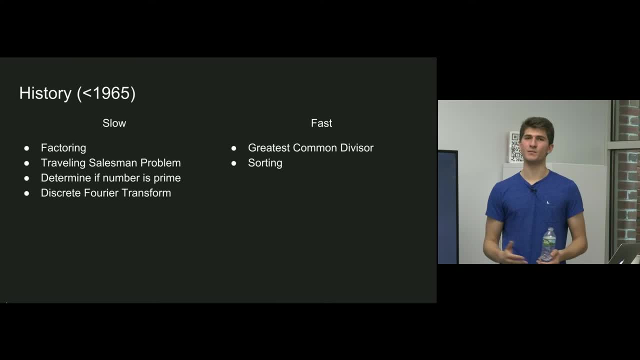 But some problems they had slow algorithms for. They were able to solve them but it just took a long time. And for some algorithms like find the greatest common divisor and sorting, we have fast algorithms like merge sort. That's worst case. running time of, I think, n log n. 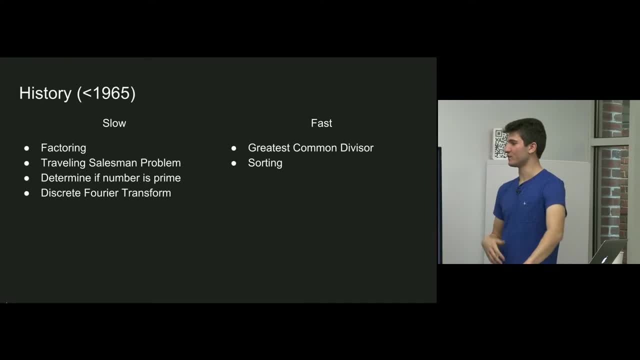 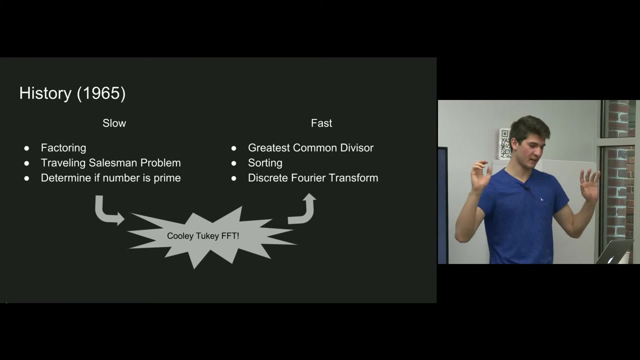 I'm going to see if I should know that. So things like that just have fast algorithms. But for some problems we just have no fast solution. And then in 1965, people came up with a solution to the discrete Fourier transform and suddenly that was in the fast category. 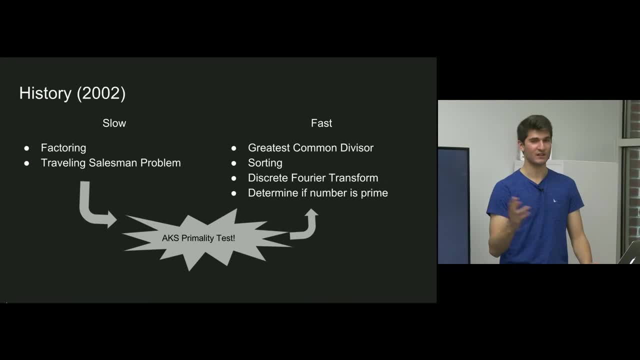 And for things like determining if number is prime. that took until 2002 for someone to find an algorithm to do that. Until it could be in this fast category, and I'll explain what a fast algorithm is versus a slow algorithm in just a second. 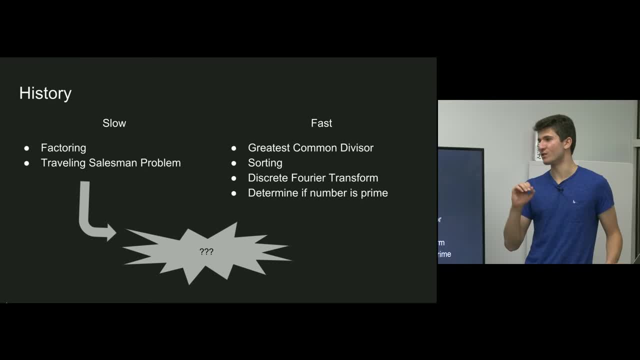 But for a lot of these problems there were just no such algorithms. There were just problems that were able to be solved quickly, And it didn't seem like we would ever find a fast solution to these problems, And so that is really the question is: will we ever? 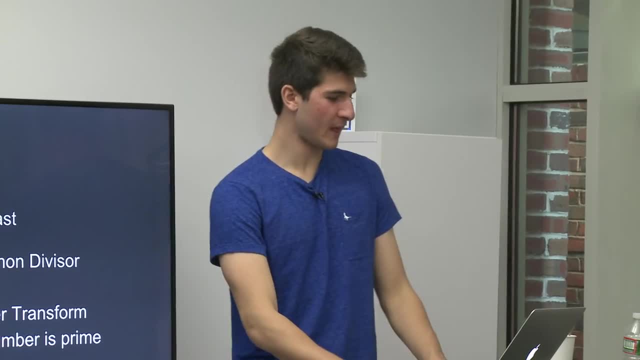 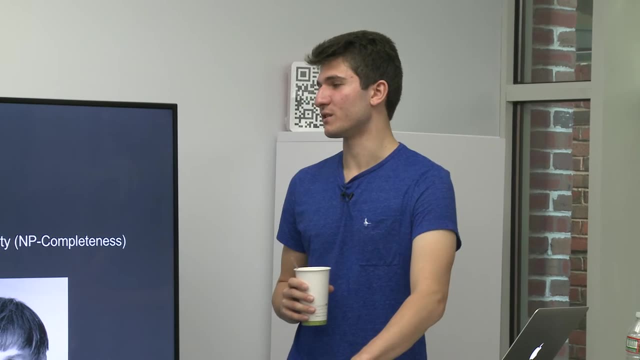 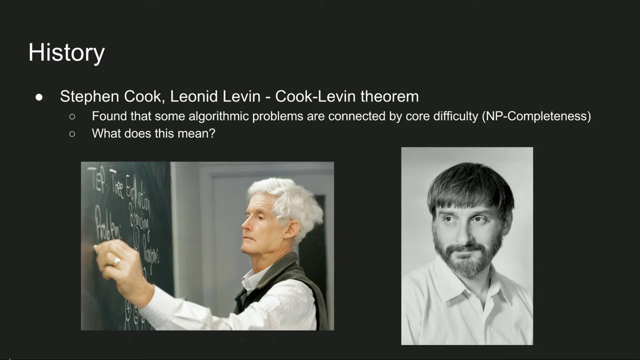 find fast solutions to these problems, And actually the answer is very unclear, Although I think one of the most important moments for this problem was a theorem that Stephen Cook of MIT and Lanoid-Livin came up with, And it basically said that a lot of problems 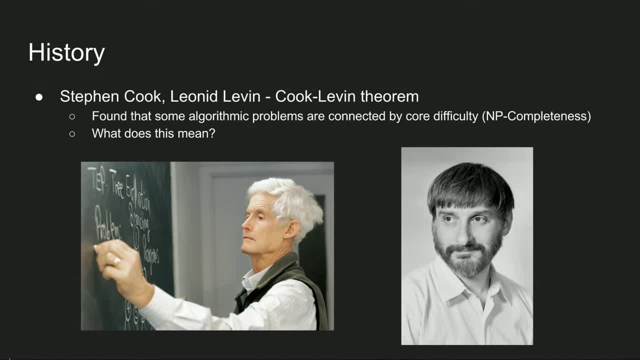 that we face in computer science are all connected by some sort of core difficulty, And what that means is that if you could have a fast solution to one algorithm or one problem, you could actually use the same algorithm to solve a very different, seemingly different problem. 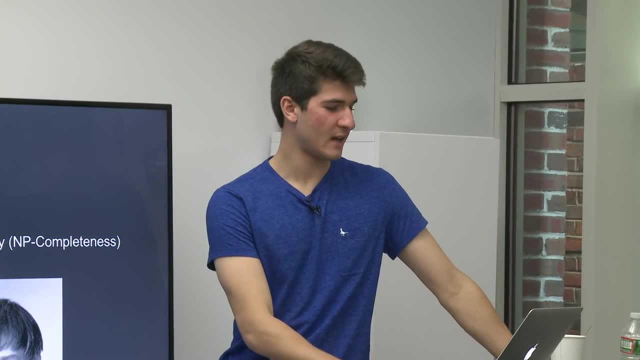 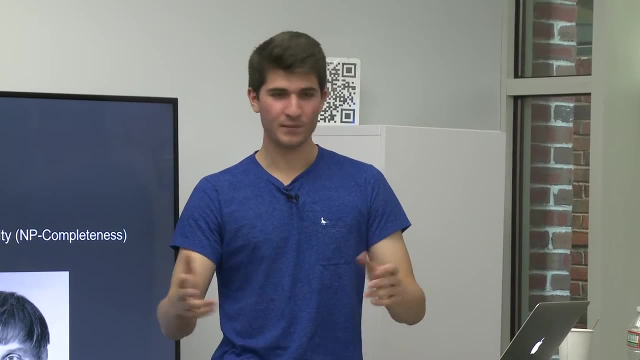 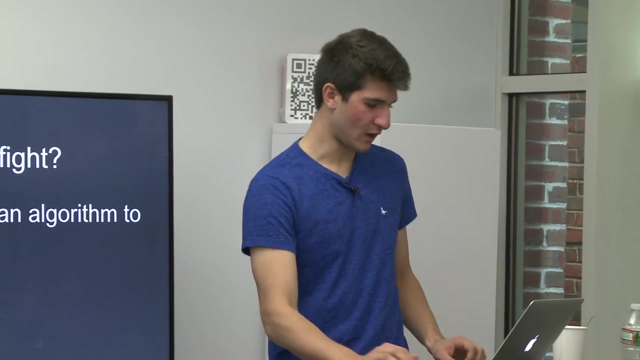 And that was a good way to categorize these problems And we learned a lot from that about complexity in general, complexity theory being the field, And we learned a lot from categorizing these problems, So I think that was a really important moment. 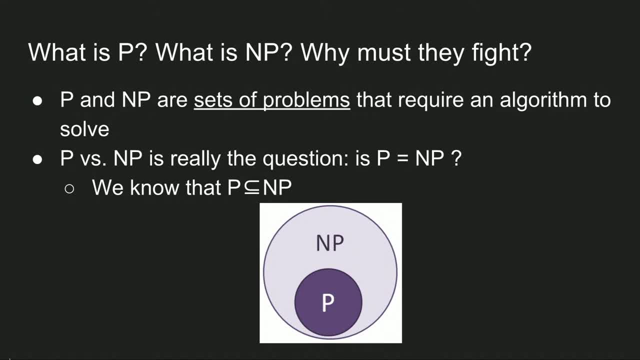 And then yeah. so let's go into a little more detail here about what p is, what is np, why are they fighting, and so forth. But at the very base of it, p and np are sets of problems. That is normally in math. we think about sets of numbers or sets of elements. 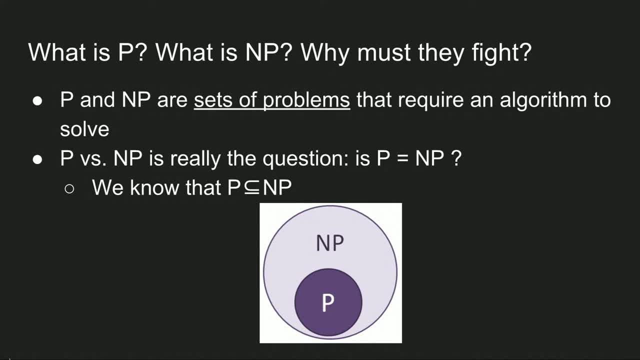 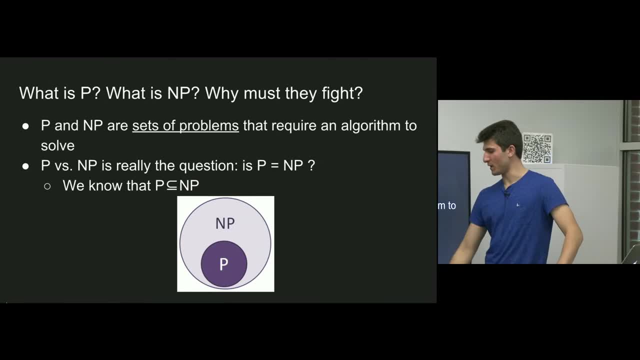 or sets of words or whatever, But now we're talking about sets of problems, And the way these problems are defined is whether or not they have these fast algorithms. So some problems, like the problems in p, actually have known fast algorithms, And some problems that are in np are at least able to be checked quickly. 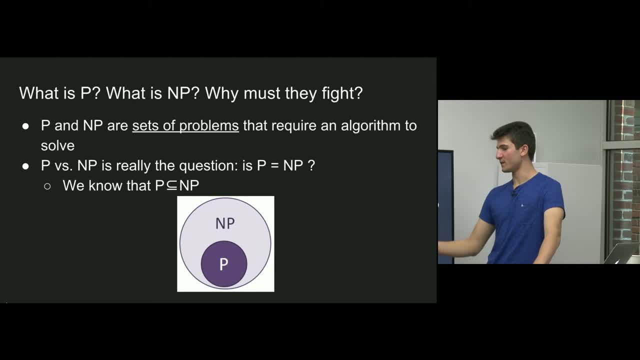 And definitely if a problem is in p, it is in np, because if you can solve a problem very quickly, it's also easy to check it, because you just solve it again, And that will all become clear, hopefully, in the next few slides. 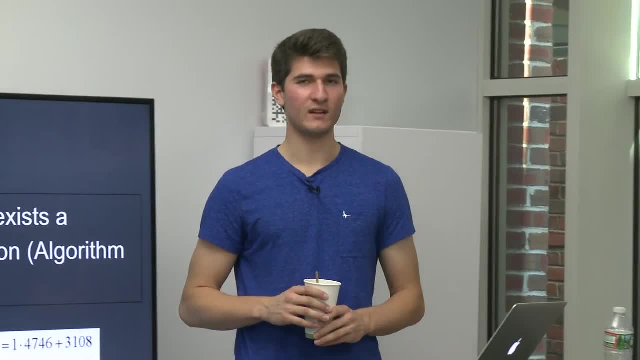 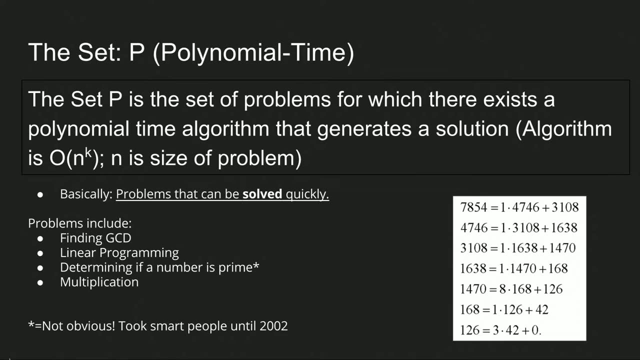 But yeah, so let's talk first a little more in depth about what is p, the set polynomial time, which is basically the set of problems where there exists a polynomial time algorithm that generates a solution. That might be a little bit confusing at first. 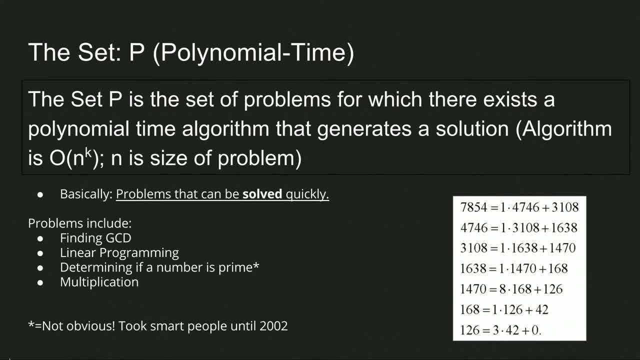 but in CS50, hopefully you learned a little bit about γ notation or worst-case algorithm runtime. sak-hoi-na-eeu mun lista is that these are the types of problems that can be solved in like a polynomial amount of time that is, like you know. it could be like 3n to the fifth plus 5. 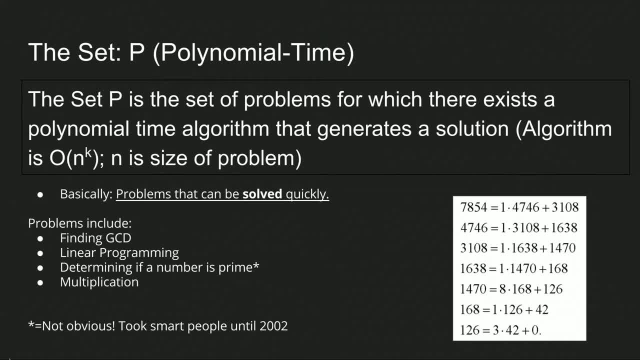 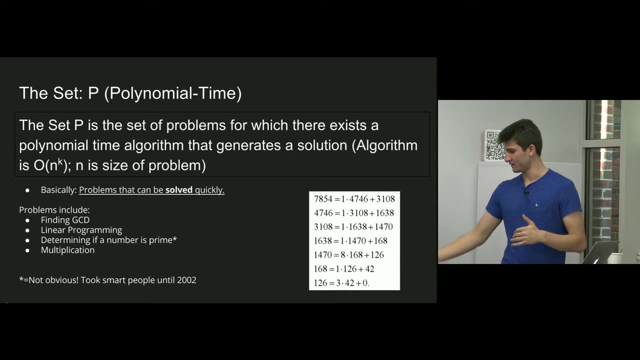 where n is like sort of the size of the problem by some definition. so these problems include, like finding the GCD if two numbers. you know, we know you have a fast algorithm for that. you know it's been known for lots, of many, many years. it's due to Euclid, excuse me, and you know you can see this is the Euclid. 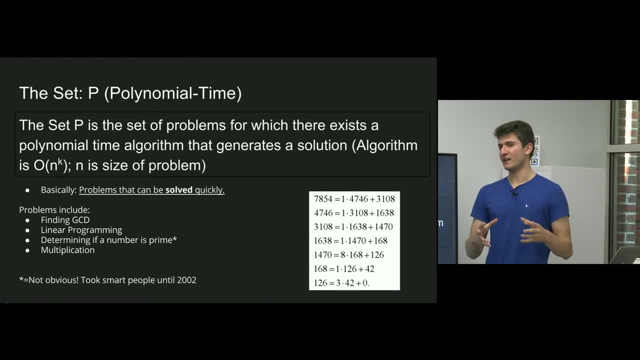 Euclidean algorithm right there, and it just is very deterministic. you just put in input and you can slowly boil down the problem into a solution. linear programming is basically like a set of equations. let's not worry about that too much right now, but that's another problem that is well known to be in P and 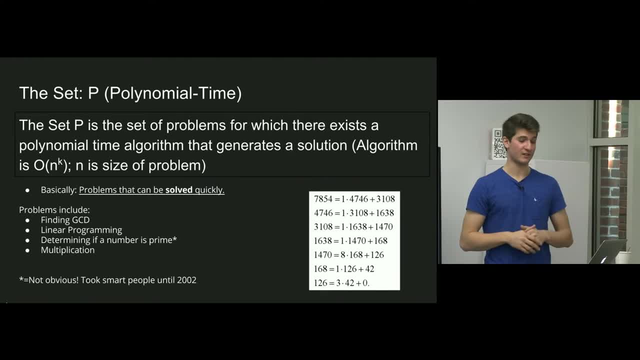 determining if a number is prime, that actually, as I mentioned earlier, that result wasn't found until 2002, but that is also in the P family of problems. um and multiplication, as you know, you probably all know the, the algorithm for multiplying two numbers. you just sort of go through one by one and that's at. 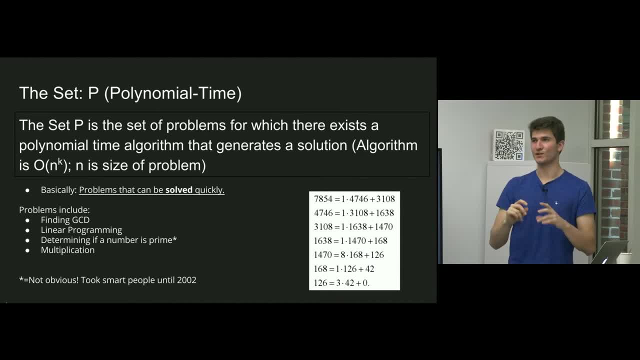 least I mean, if you multiply every digit by every other digit, that's sort of like n squared. then you add them up, so it's sort of a most n cubed. but crucially, these albums, these- excuse me, our algorithms aren't like 2 to the n or 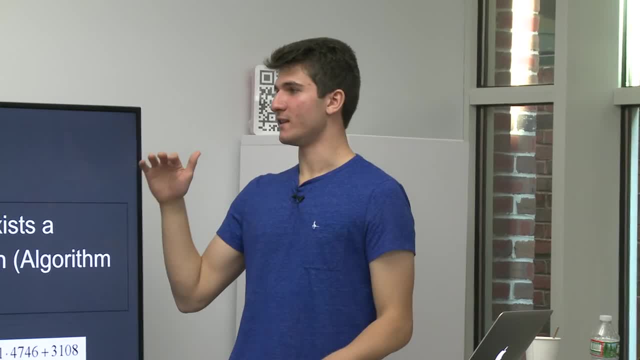 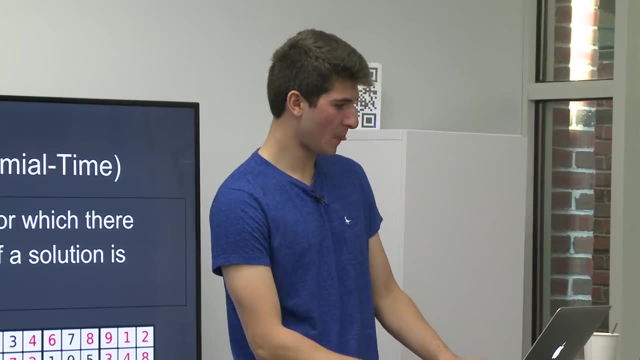 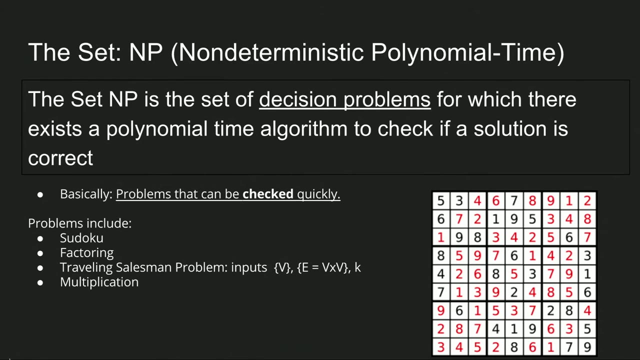 something exponential. so that's what makes them in this category of P. yes and yes, let's move on a little bit to the set NP, which stands for a non-deterministic polynomial time, which is sort of like a way of saying: well, they have polynomial algorithms to solve them, but like they're non-deterministic, which? 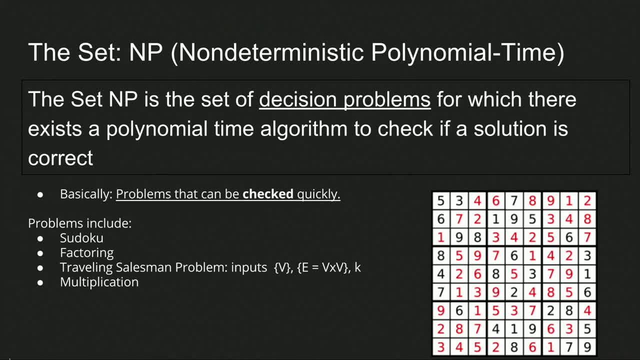 means you just sort of have to guess or like use an infinite number of computers before you can solve them in a polynomial amount of time. but the way these are defined formally and before we talked about problems that can be solved quickly. now we're talking about problems that can be checked. 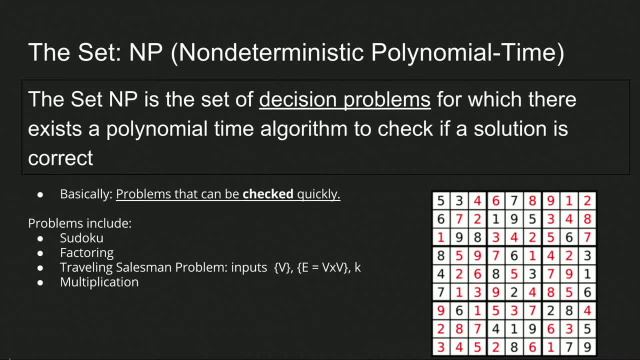 quickly, and what that means is it's a set of decisions, problems- and I'll explain what that means just a second- for which there exists a polynomial algorithm to check if a solution is correct. so before we're saying I'm giving you a problem, tell me. you know a solution. you know in some, in some. 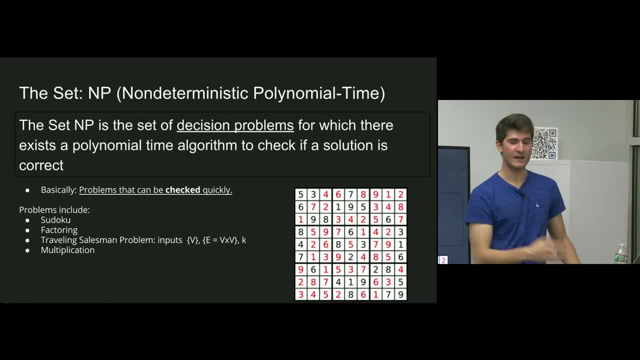 definition of the solution. and now I'm saying here's a problem and a solution and I want you to check the solution. so does a set checking take a polynomial, polynomial amount of time? and so these problems are- I guess problems included in this set are like Sudoku, because you 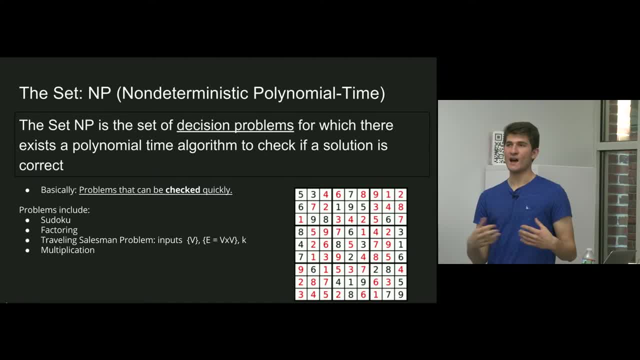 know it. if I give you Sudoku board and said this is solved, how fast would it be for you to check if it was solved? it actually wouldn't take you that long. you'd probably just go through every row column and you know 9-by or. excuse me. 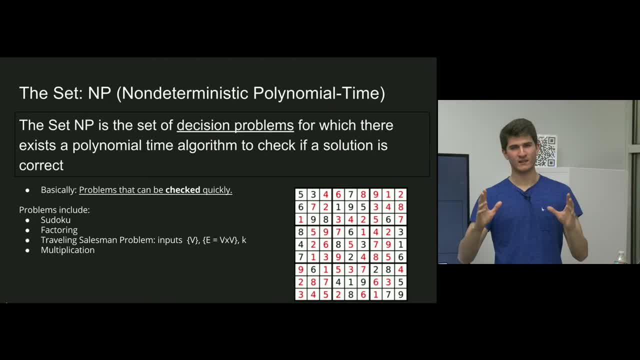 3 by 3 square to check, and that's you know what, like n cubed, but crucially it's not something like N squared. so it's just, you know there's this problem. So these problems are B and C because there's a set of easy to solve problems. see, if you don't know exactly what the answer is, you can go to C next, and you know. so you do have a set of, you know there's a set of, you know there's a set of problems that you can go to. so that's a couple of problems that you can. 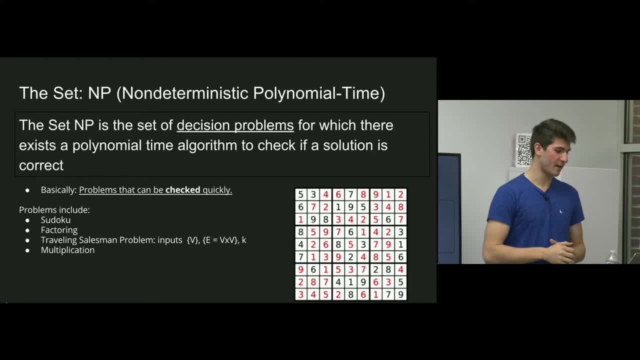 n or 9 to the n, which would be an exponential amount of time. And another problem is factoring. So it's easy to check if a factor is or if a factorization is correct. You just multiply the numbers and then you. 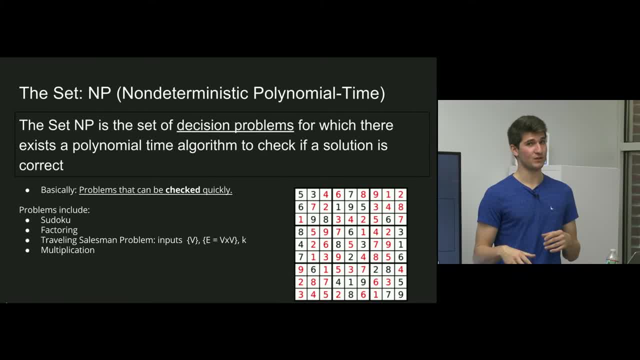 can see if that factorization is correct. Much harder problem to factor the numbers, by the way, And traveling sales problems- is an example of a famous NP problem where you're given a graph with vertices and edges, And we'll get into a little more about graphs in just a second. 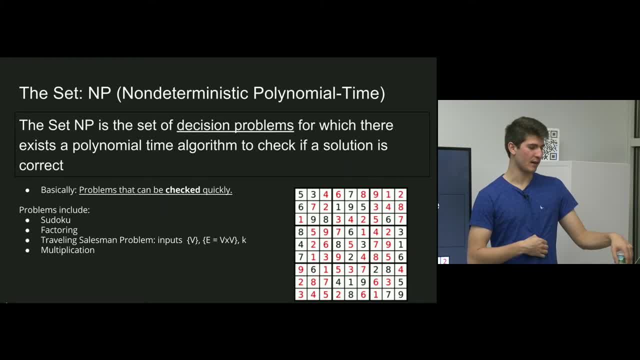 because those turn out to be really relevant to NP problems and thinking about them. But again, multiplication: I thought we just said that was a P problem. Well, if something's in P it's also an NP, Because if I said, well, what's 51 times 3?? 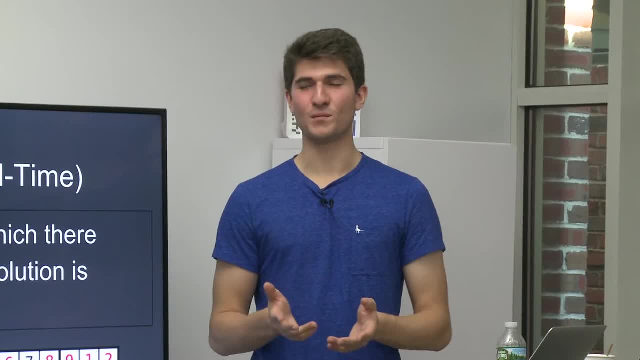 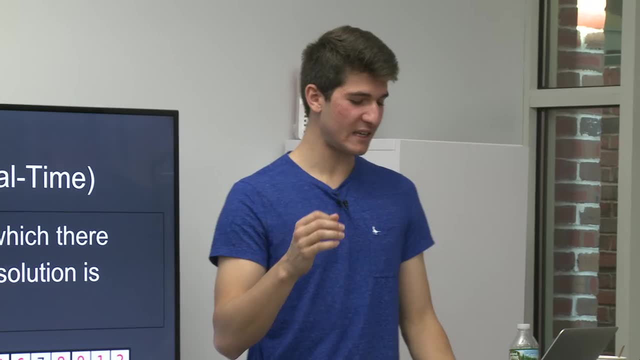 If I said 51 times 3 is 153, well, how would you know? I mean, you'd probably just check it yourself and multiply it yourself, And of course that's, as we described, a P algorithm. So that has a P algorithm to check whether or not my solution's correct. 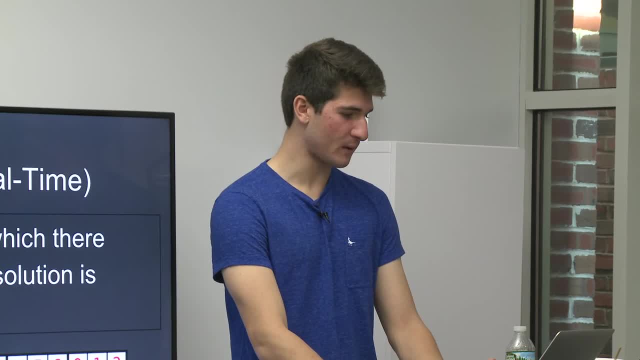 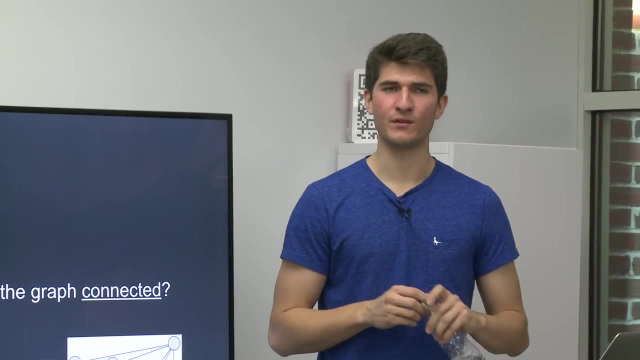 That's how you know. it's in NP. So we've talked about P, We've talked about NP. So now we have a couple examples here that maybe give you a better grasp of how to think about different problems. So sorting a list: is that in P or NP? 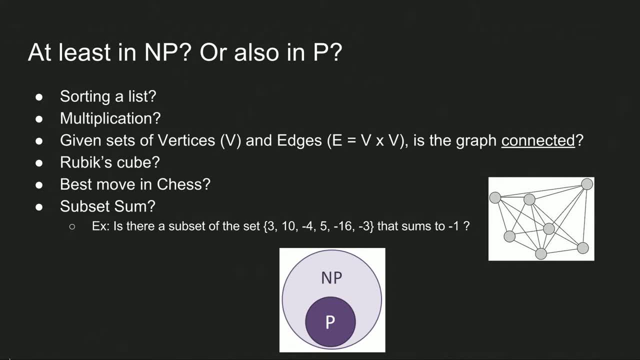 Well, you talked about sorting and the running time of those in CS50. Hopefully you know that for a lot of sorts that's like n log, n Or like n squared, I think, for a quick sort. But those all have polynomial time algorithms. 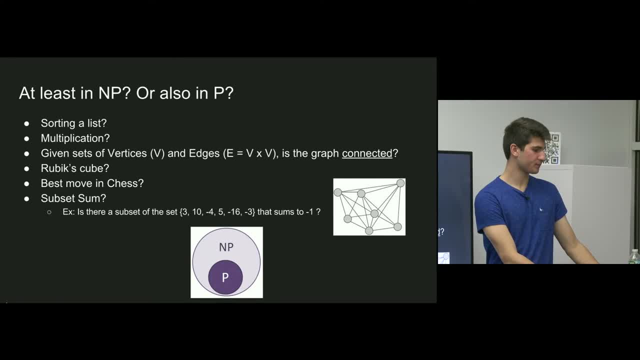 So those would be in P. also in NP Multiplication we just described P algorithm right. It's like something like n cubed And then, given a set of vertices and edges, is the graph connected? Is that P or NP? 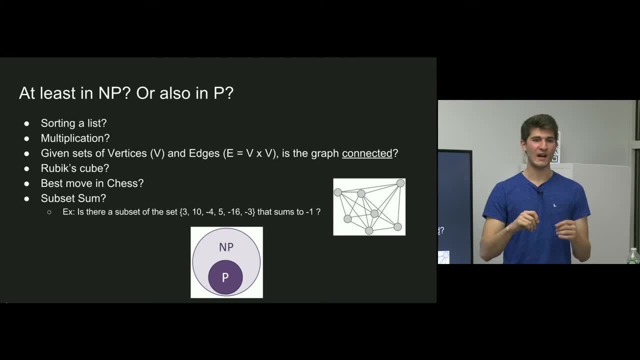 Well, I mean, you just start at a point and you traverse until you have seen all the edges. If you haven't seen, excuse me, all the points, If you haven't seen all of the vertices, then you know it is not well connected. 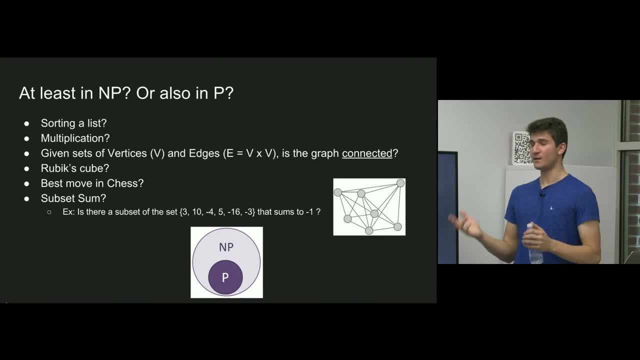 And another example would be a Rubik's cube. First of all, is that in NP, That is, is there a way to check if the Rubik's cube is solved? Well, yeah, it's pretty easy. You just check if all the faces are solved. 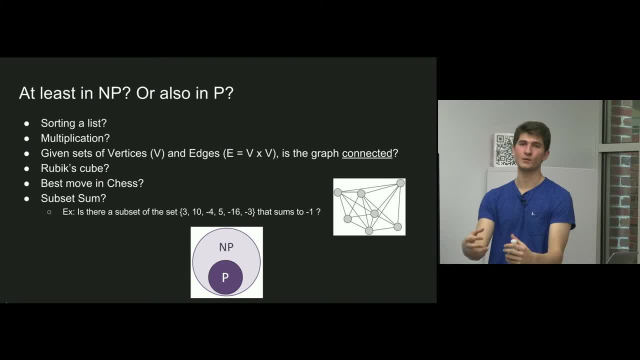 But is it in P? Is there a polynomial time algorithm to actually solve the Rubik's cube? That is actually a little harder to think about, but it turns out it is actually. Computers can do that fairly fast. And what about the best move in chess? 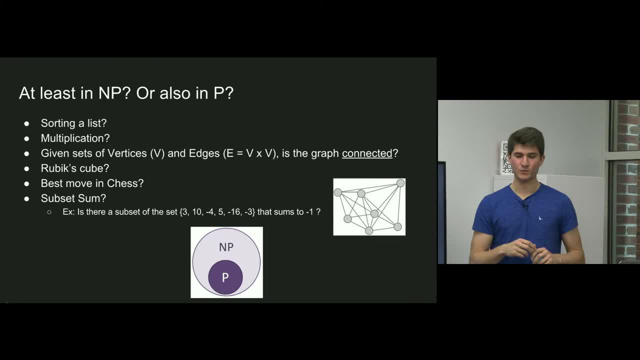 Is that in NP? Well, if I told you that this is the best move in chess, could you check that it's the best move in chess? Probably not. I mean, I think you'd have to go through more calculation to determine if that was the best move. 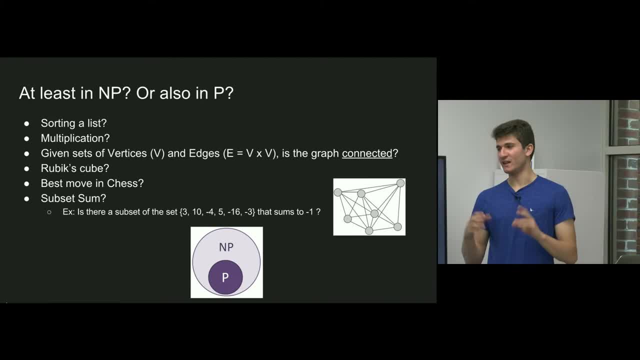 And that problem actually is not in NP or P, That's in its own class called exponential time, where it takes exponential time to even check if a solution is correct. And then there's problems like a classic NP problem is like the subset sum problem, which means given a set of integers, 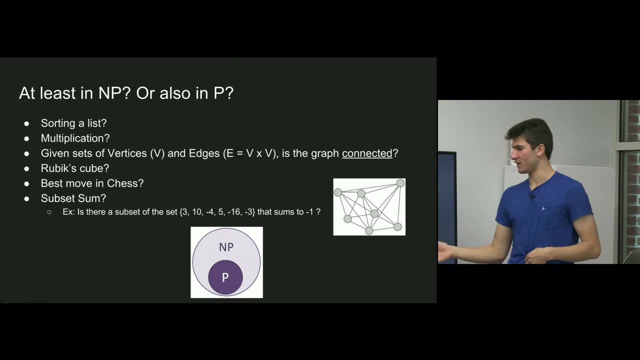 say I'm asking: is there a subset that sums to negative 1?? And in this case you could just look at it And if I gave you a subset and said these sum to minus 1, it would be really easy to check. 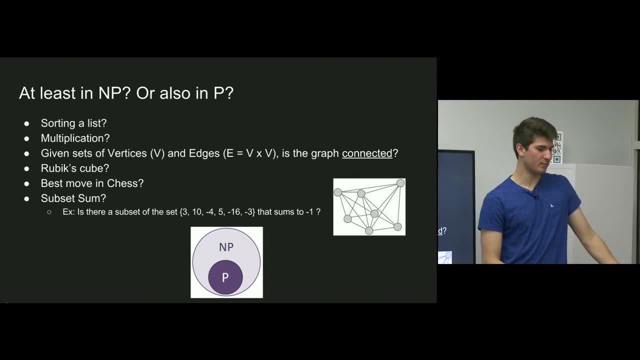 I mean you just sort of sum them up and they sum to minus 1.. But solving that problem actually isn't very easy And there's some sort of exponential time, There's some exponential checking that you have to do to determine if there is such a subset. 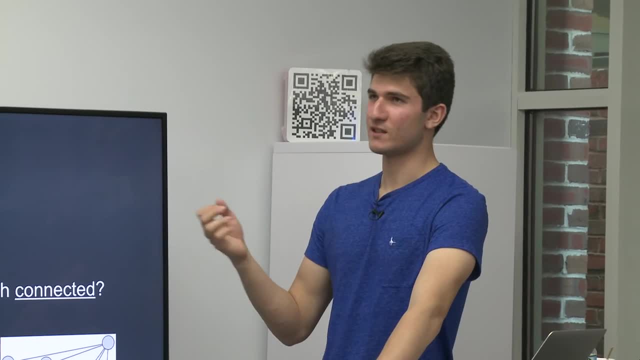 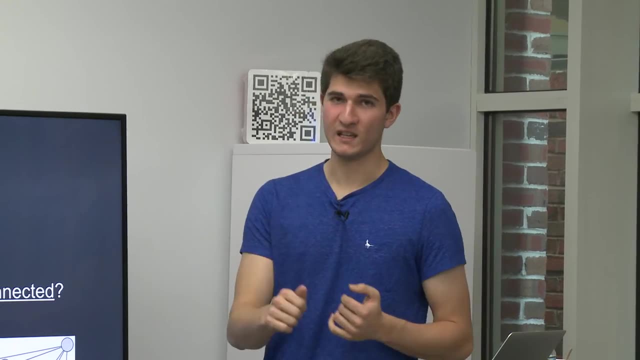 And if you think about how many subsets there are, two to the n subsets, I believe, where there's n members of a set. So you kind of have to check a lot And that's a good indicator that it is not in P. 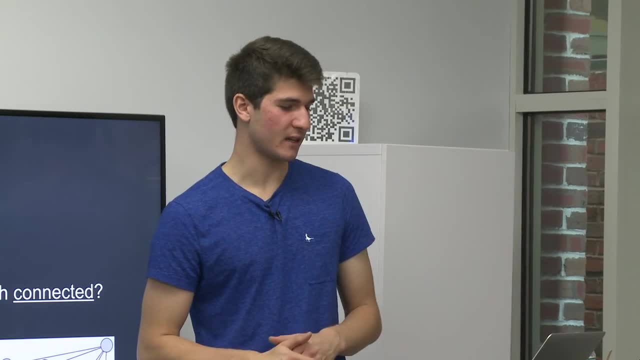 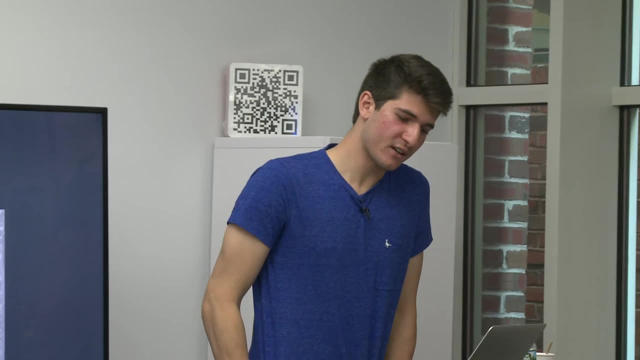 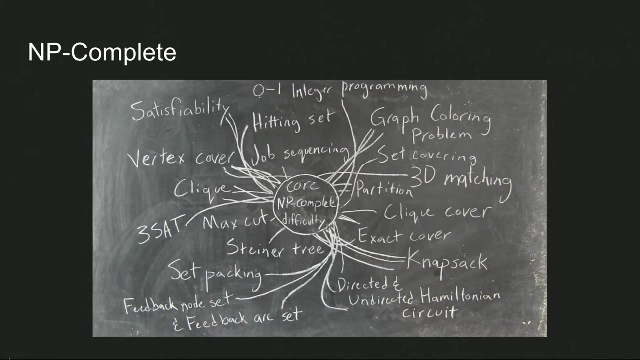 But in this case it is as we showed in NP, because it's easy to check. So I was talking to you before about NP-complete And this is sort of one of the most important concepts to understand when talking about P versus NP problem. 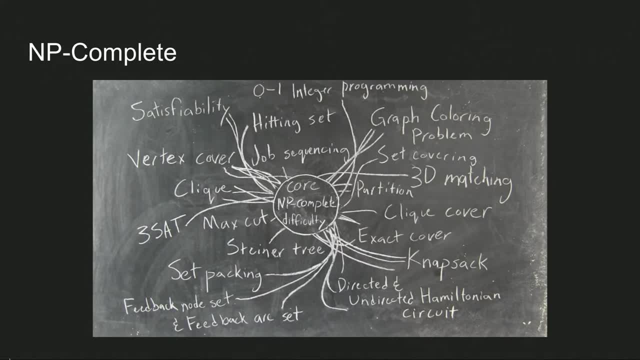 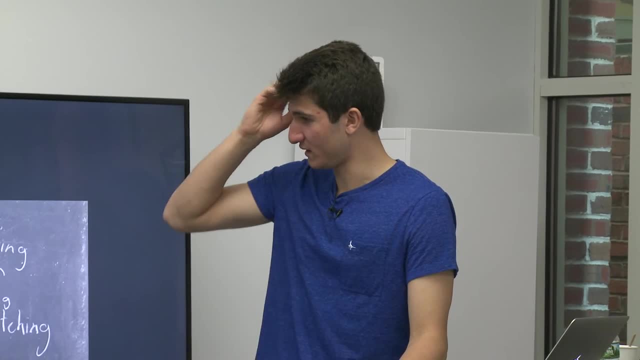 Basically what this means- and this is related to the Cook-Levin theorem that I was talking about earlier. it essentially says that all of these problems- and this is an example of a bunch of NP problems- they're all sort of connected. 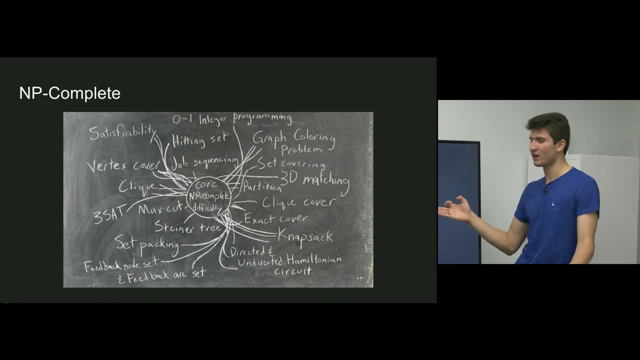 Where, if you have a solution, say, to the graph coloring problem, you can use it to form a solution to the click cover problem, or to the hitting set problem, OK- Or to the yadda yadda. You can basically form one solution into the other. 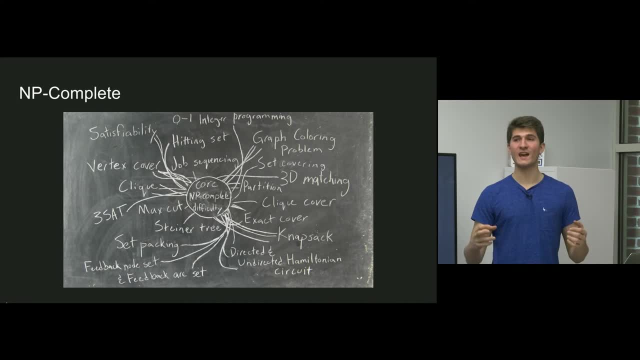 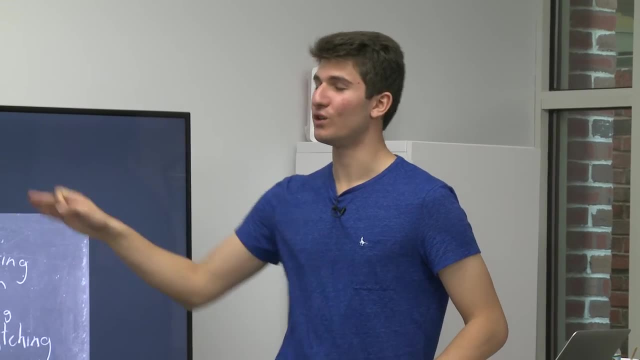 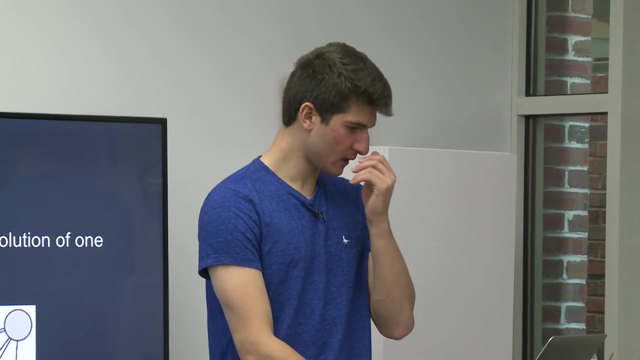 And that's really powerful Because if someone one day finds a polynomial time algorithm to do one of these problems, that means they can find a polynomial time algorithm to do all of these problems, because they're all sort of related and can be converted to one another very quickly. 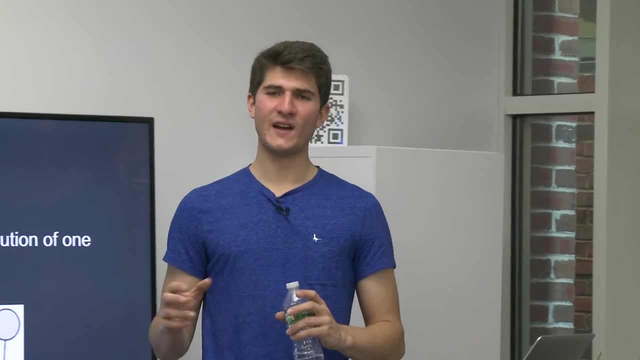 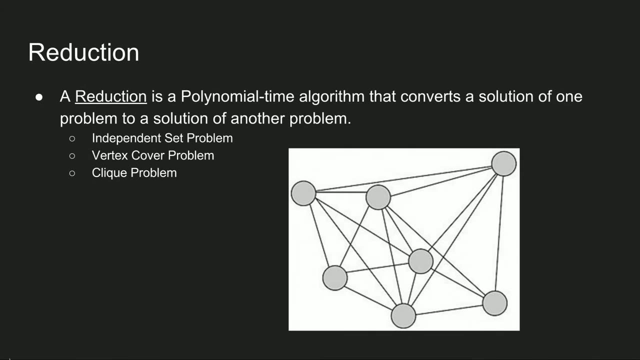 And I sort of glossed over detail there, which is how fast can these algorithm solutions be converted to one another? And that has to do with reduction, And I just want to talk about this for a second because this is sort of one of the more core concepts that 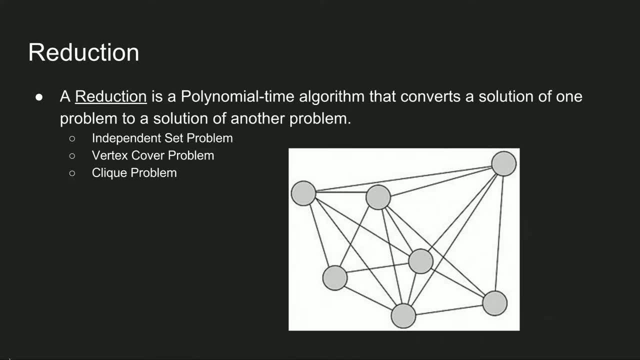 is involved when proving these things, And this is actually what computer scientists have to do when they talk about: are these problems NP complete? Are these problems related by some core difficulty? And what it means is basically a reduction is a polynomial time algorithm that converts a solution from one problem. 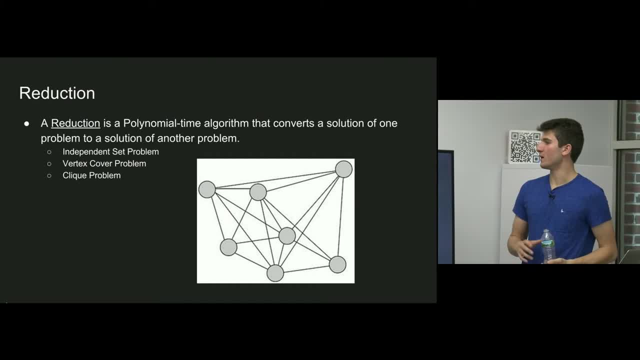 to the solution of another problem, And I'm going to be talking a little bit about three particular computer science related problems, which are the independent set problem, the vertex cover problem and the click problem. Independent set problem has to do with basically given a graph. 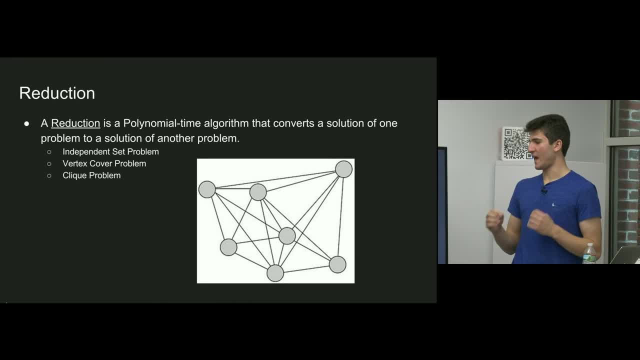 like the one I'm showing in the slide. are there a set of k vertices such that no two of those vertices are touching or related by an edge? The vertex cover problem means: can you give me a minimum set of vertices that That covers all of the edges? 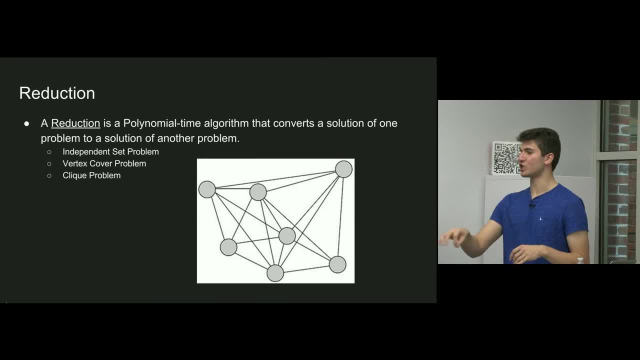 That is, that all of the vertices are touching every one of the edges in the graph. And then the click problem. I don't know if it's click or clique. Some people say clique, But it's related to the colloquial sense of the word click. 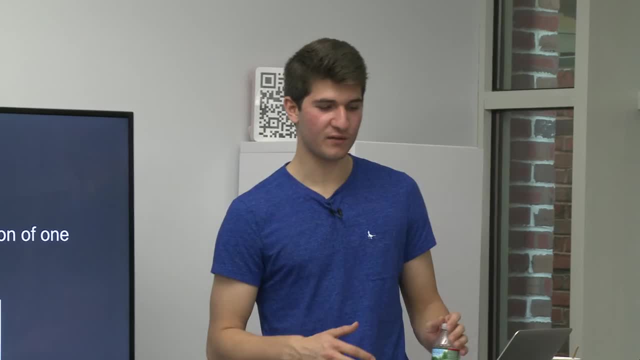 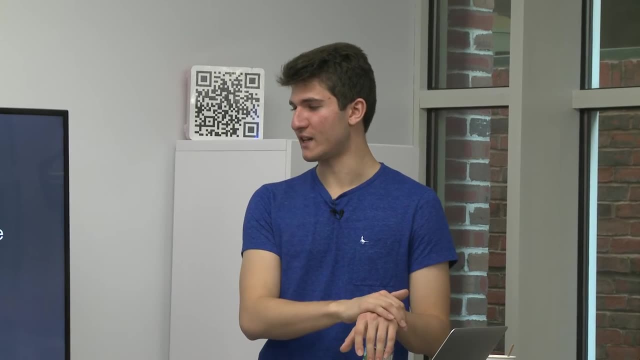 which is like a friend group. Is there a friend group, essentially, in this graph, where every single person in the graph, every person represented by a vertex, The vertex is connected to every single other vertex in the clique And in this case you can see there is actually. 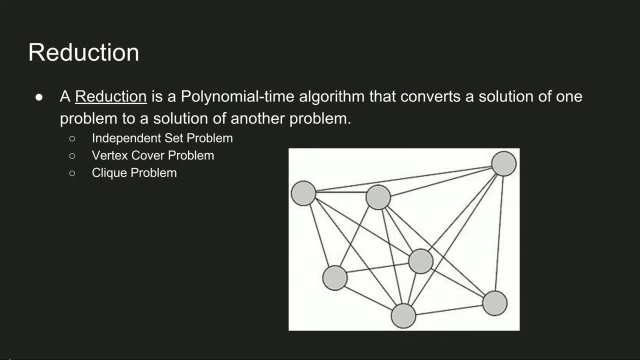 a five clique in the bottom left of these five vertexes are all connected to each other, And so that makes them what's called a five clique. So these are three problems that I'm going to go into in detail just a second, And I'm going to show you that they're actually all sort of the same problem. 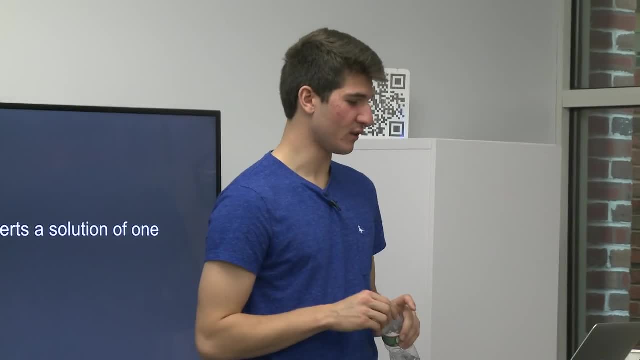 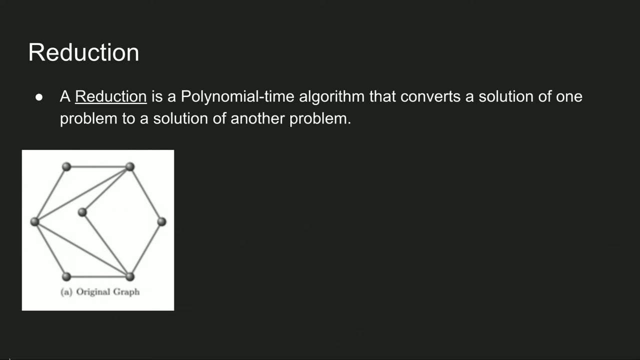 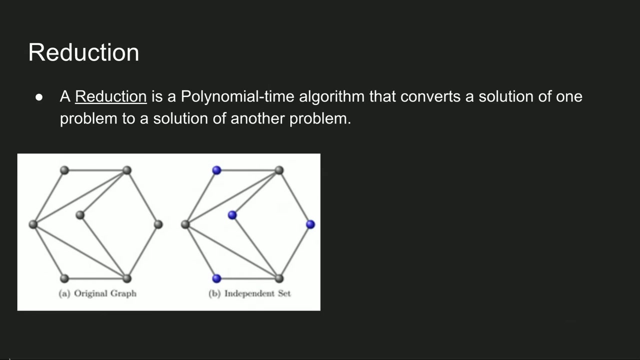 And solving one can actually give you a solution to another. So let's take the example of this graph Again. graph, just generally, is a set of vertices and edges connecting them, And this is an example of an independent set. So how do we get this? 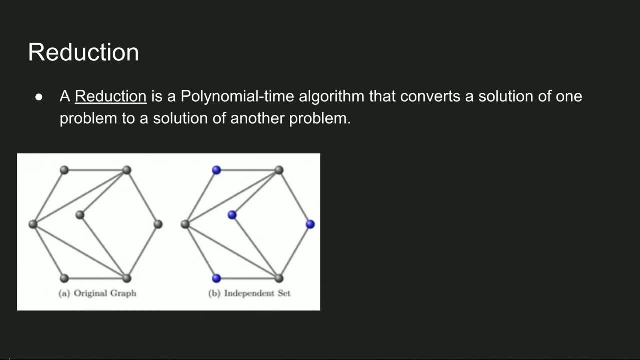 If I just said to you: give me four of these points, such that no two of them are related by an edge, then this would be the solution. Great, So how long did that take? Well, if it were a big graph, it would have. 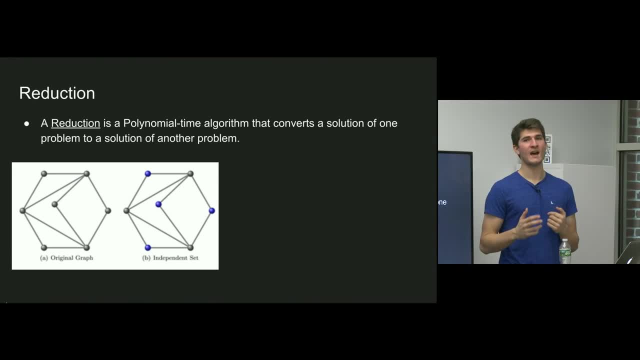 taken some sort of exponential amount of time. There's no polynomial time, There's no algorithm to do that. But if we are able to get a solution, we can use it to solve some other problems, And in this case we can use the independent set. 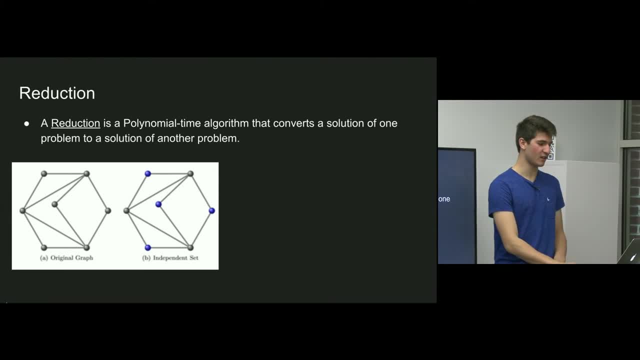 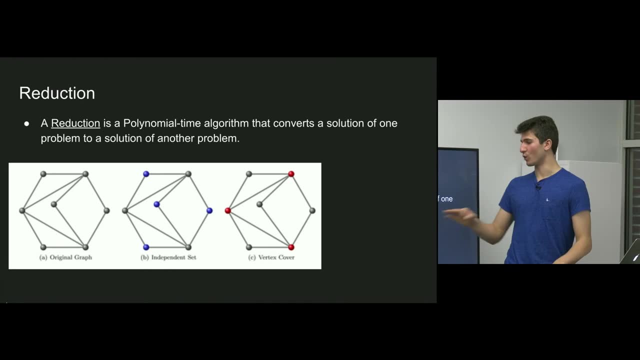 to solve the vertex cover problem. How do we do that? Well, we just consider all of the vertexes in the complement, So basically all of the vertex that weren't in the independent set. consider those to be in the vertex cover. 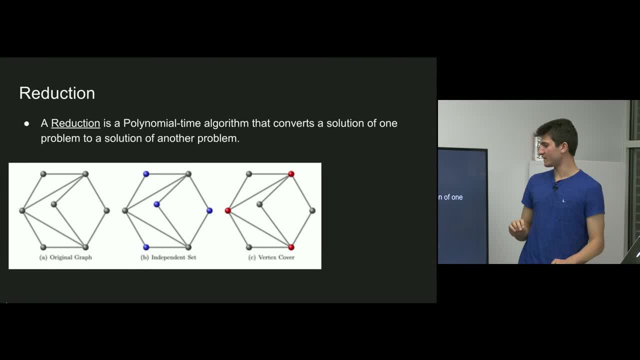 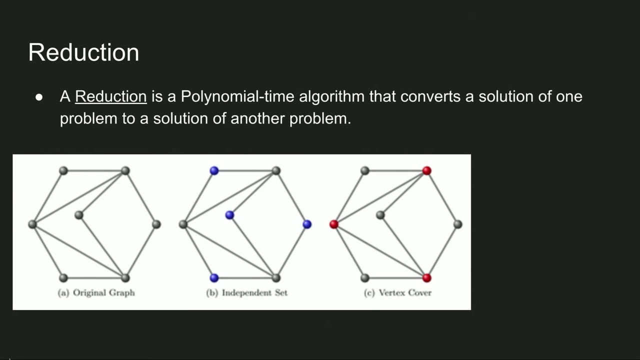 And these have the property that every single vertex is related to every other edge. All right If I'm explaining that correctly, but every vertex in the vertex cover is touching every single edge, And in this case you can hopefully see that, And so we just created out of nothingness. 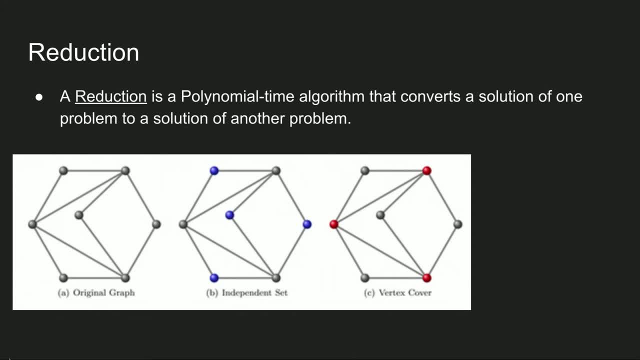 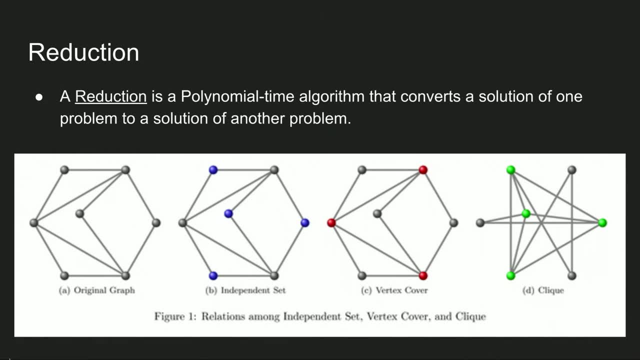 a solution to vertex cover from a solution to independent set, And we can even take it one step further with clique. The way you do this is you consider the points in independent set or the graph of independent set and then take the complement of the edges which 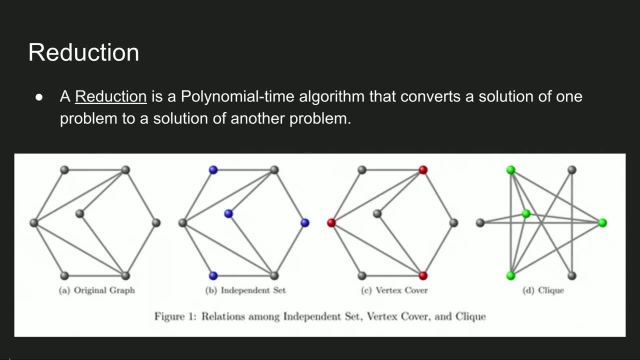 means that every compli-, Every edge that doesn't exist already, you fill it in, And every edge that did exist, you get rid of it, And what you're left with is this graph And all of the points that were originally in independent set. 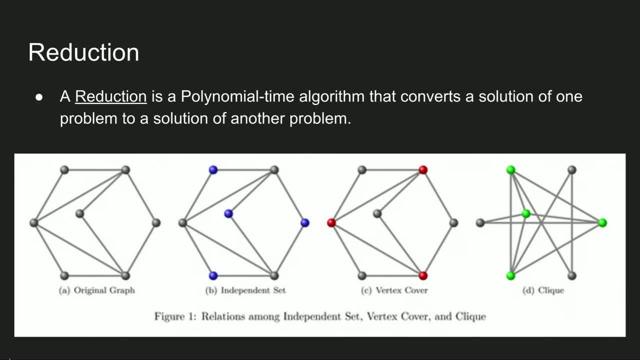 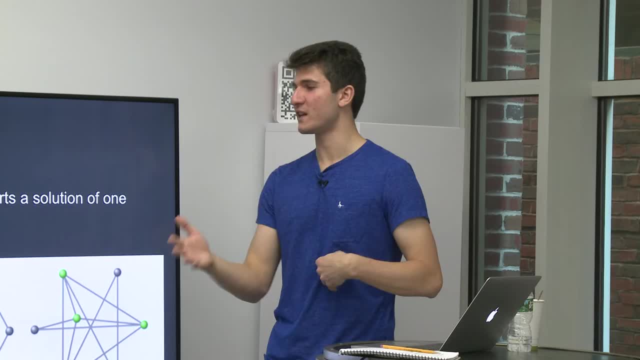 are now a clique, in this case a for clique- for this new graph. So it took a long time to create a solution to independent set in exponential amount of time. Now that we have that, we're able to create solutions to other similar problems. 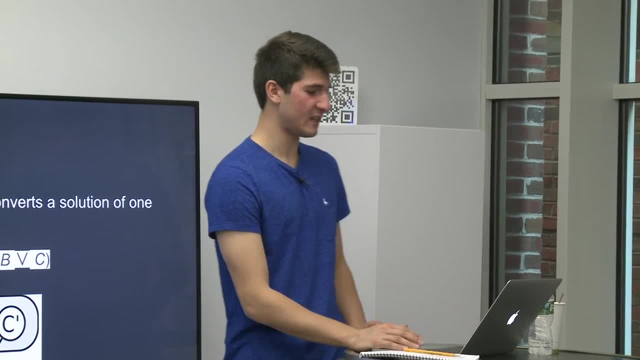 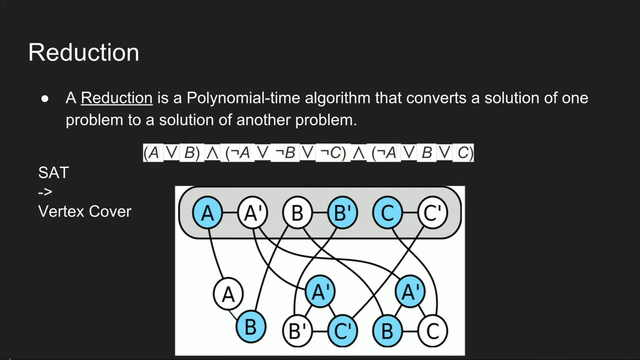 And it turns out there's a wide range of problems. There are problems that are related, even problems not really seemingly related- to graphs at all. So this is sort of what's called the satisfiability problem, Given a clause or a basically logic clause, where each of these variables 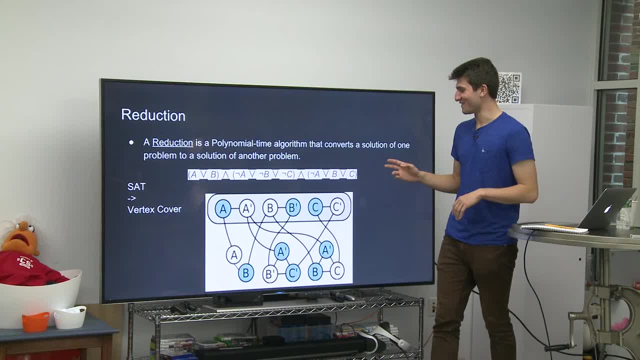 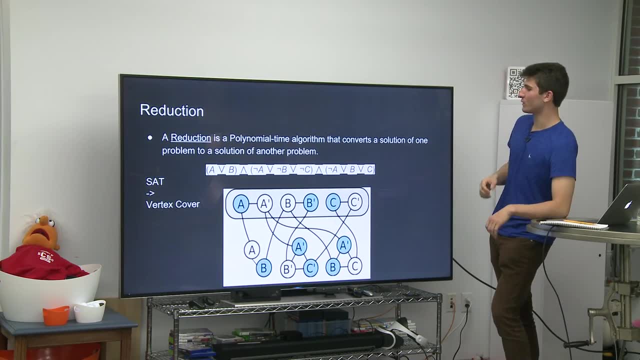 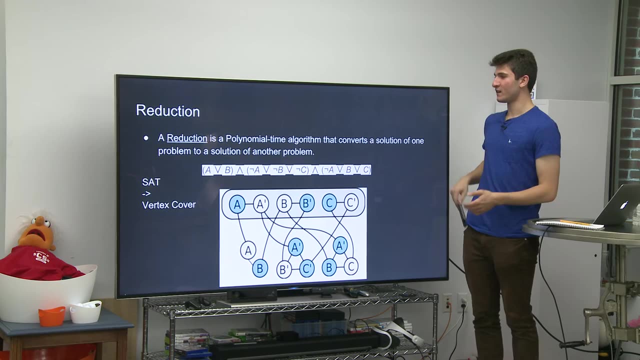 I don't know if you can see where I'm pointing in the video, but these are all basically variables that are either true or false, And so what the satisfiability question is asking is whether or not this clause has a truth assignment, That is, there exists an A and B such that this all becomes true. 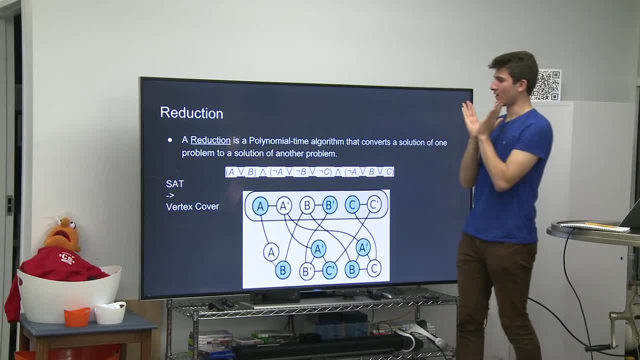 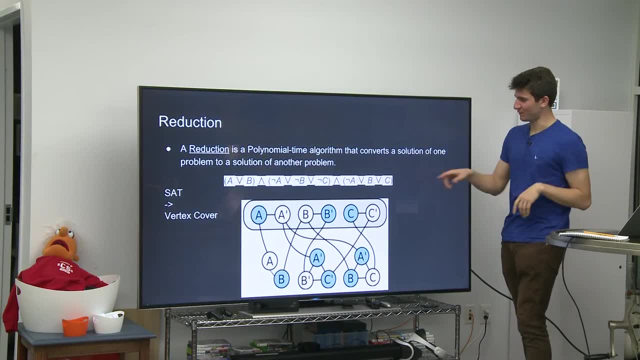 And for those who don't know, these little downwards carrots are ors and the sort of upward carrots are ands, And the little- I don't know how you call it- the little sideways dashes are nots. so like the opposite. 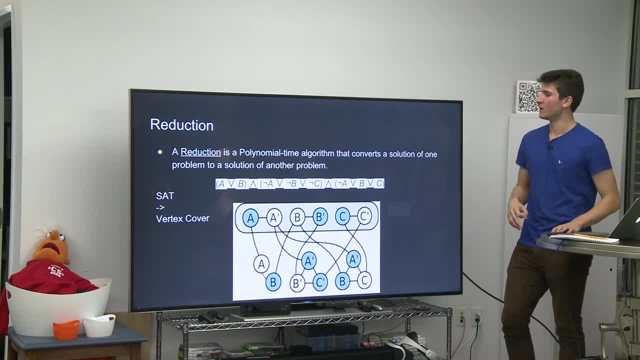 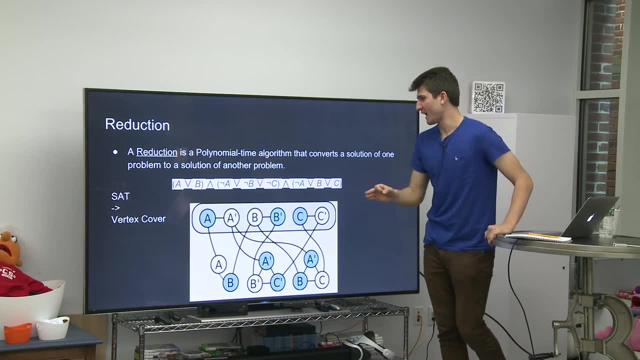 If it's true, it's false. If it's false, it's true. So the question is, does this have a truth assignment? And maybe you can just eyeball it and say: well, actually, if A is true and B is false and C is true, then this statement can be true. 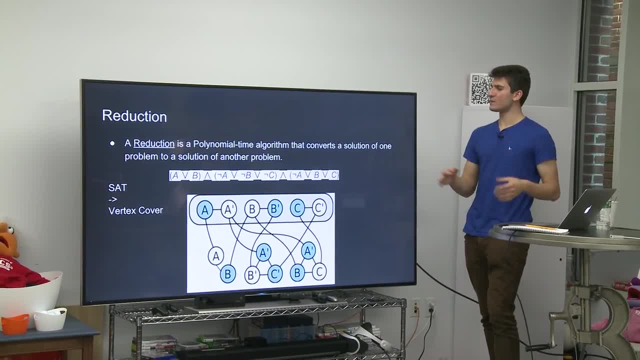 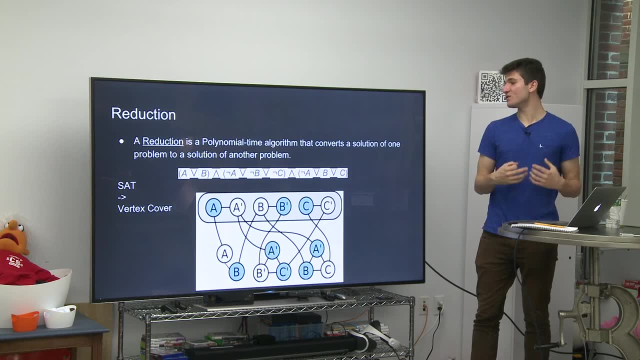 And indeed that is the case. So how do we reduce, how do we take that solution and turn it into a solution to say, the vertex cover problem? In this case, all we have to do is create this graph, And there is an algorithm to create this graph. 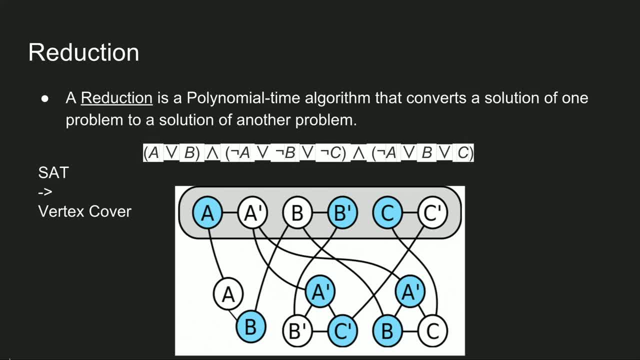 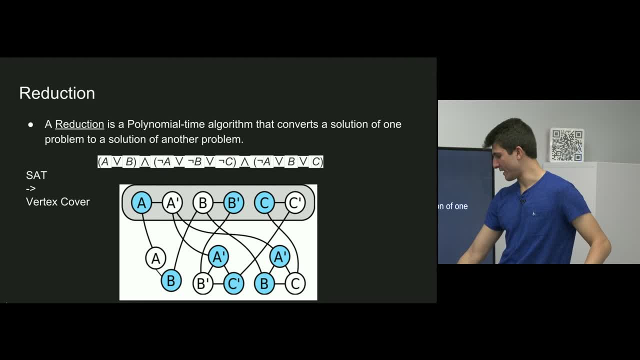 And what it does is you. basically, I don't know if you can see this, but every clause of the original Statement up here turns into two variables at the bottom of this graph. So you have AB turning into AB down here, not A, not B, not C. 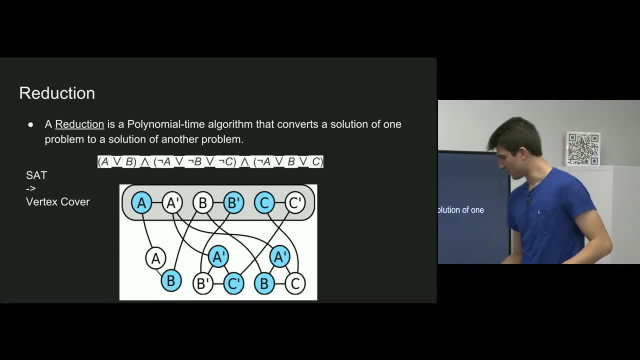 turning into these three points down here, And then not A, B C, turning into not A, B C And then finally you just take every A and its complement up here. Now let's say we have the solution A, not B C. Then 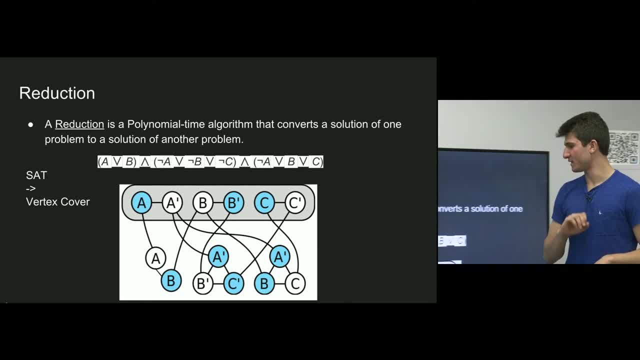 basically, you want to color these A, not B, C- on the top line And then you want to connect every single element to itself. So not B goes to not B, B goes to B, A goes to A, not C to not C. 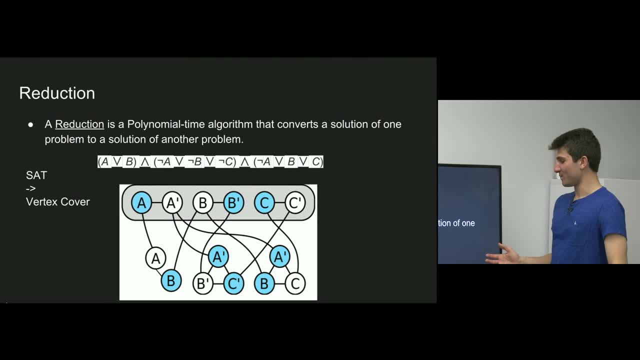 and that's that. The point is that basically, oh, did I miss something? So then you basically color these based on. there is a relationship- I'm actually blanking on it right now, But basically there's a way to color these. 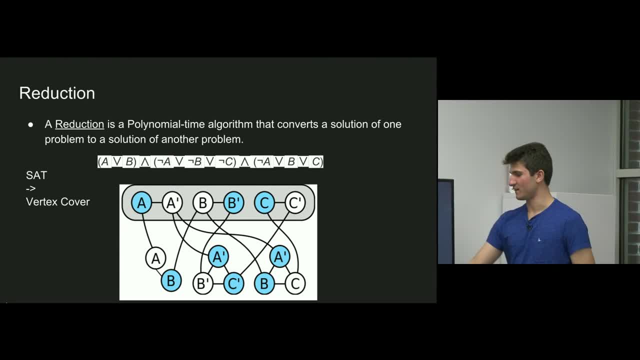 And basically, when you color the A, not B, C, and then the B not A not C, B, A, in the bottom, that creates a vertex cover And so you've used a solution. You've used an algorithm that creates a solution from the satisfiability. 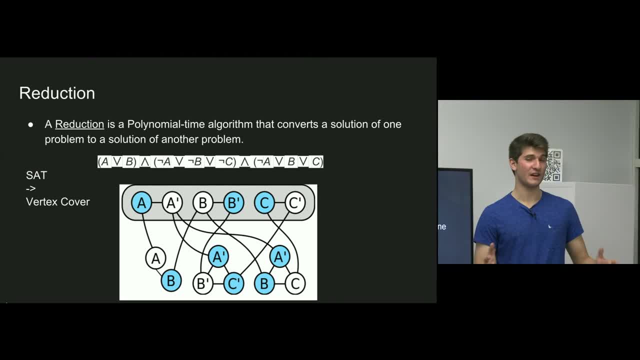 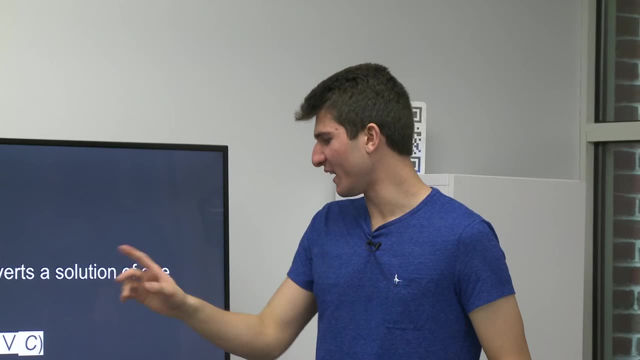 into the vertex cover. that is actually very powerful And that's what's called a reduction. I know that was a little bit involved and I'm still trying to figure out how these are related. But basically A, not B, C, Yeah, so I think what it is. 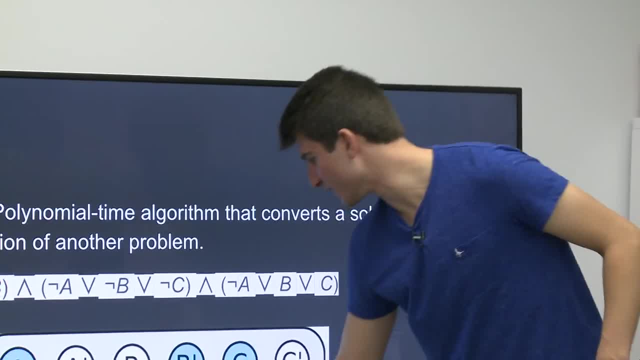 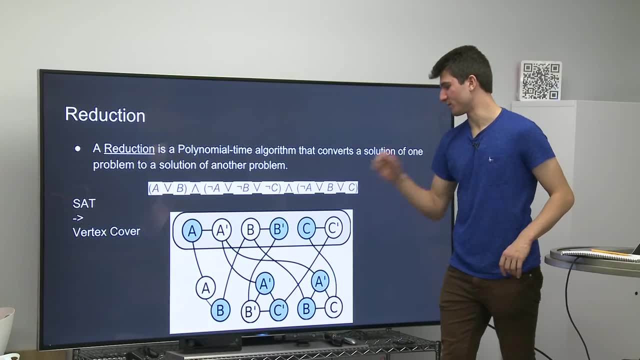 is, if it's A is colored here, then you color all the not A's in this bottom graph. And if not B is colored here, then you color all the B's in this bottom graph. And again, if you color C here, then the not C is colored here. 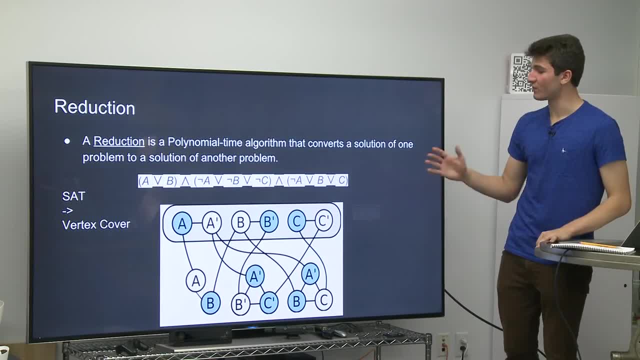 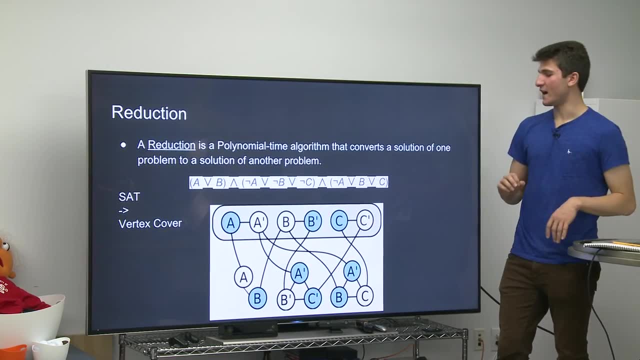 And I think using that algorithm you can create a solution to vertex cover. Why is this a solution to vertex cover? So that's one thing I didn't mention. It's that all of the colored things are covering every single edge, That is, every single blue node here is connected. 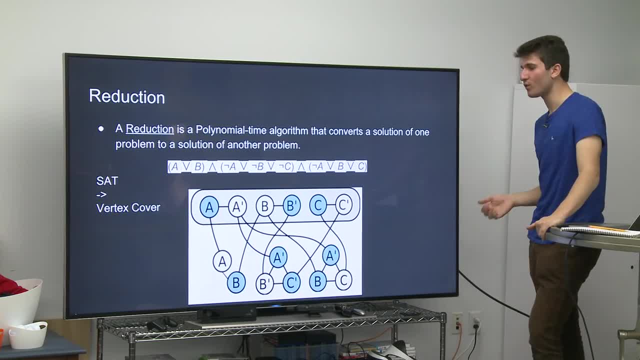 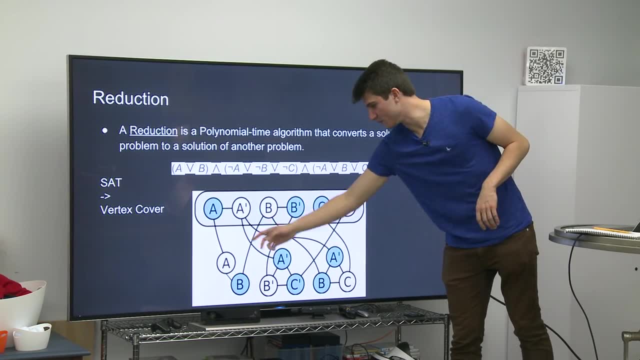 to every single edge in this graph. Also, as we discussed before, vertex cover is related to independent set in the complement. So if you consider all the white nodes in this graph, they form a independent set where no two of the white nodes are touching. 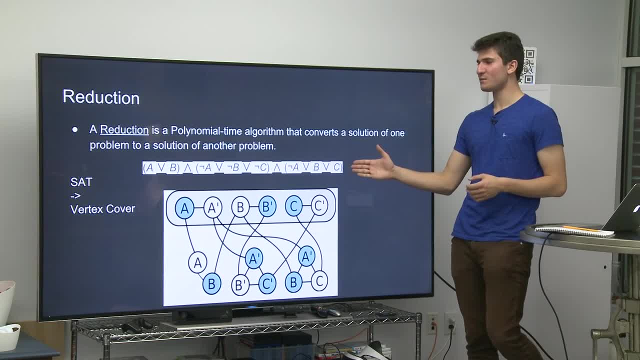 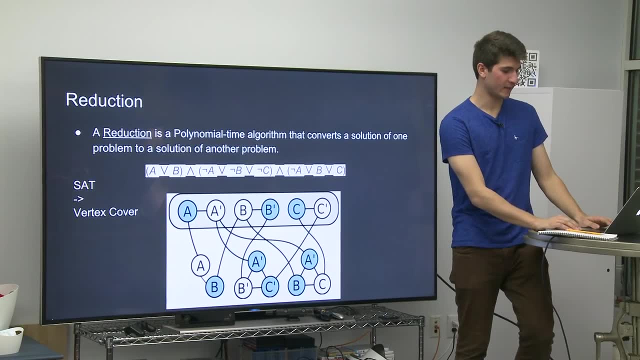 So now we've created solutions to two of these problems from a seemingly completely unrelated problem, which is the satisfiability problem, And that's actually really powerful when considering these type of NP problems. Sorry, that was a little bit wordy. Hopefully you got something out of that. 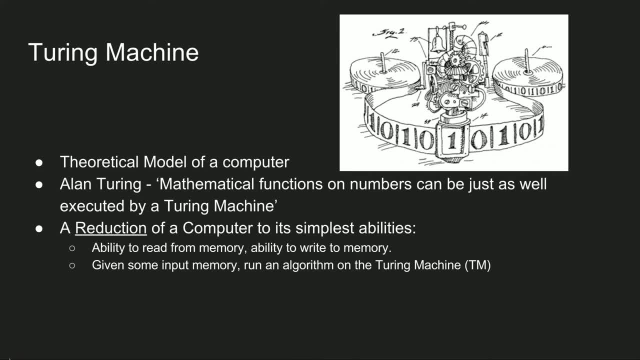 Let's go on to more fun. things like the Turing machine Way more fun. Of course, this is due to Alan Turing, the man who needs no introduction, But basically this was his theoretical model of a computer in its simplest form. 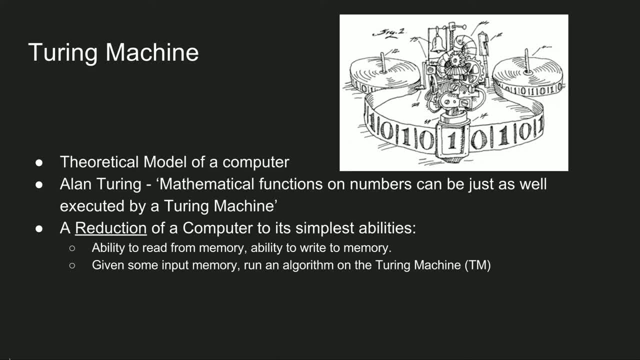 which is basically, you can do this. It's just something that runs, an algorithm. I think this image helps to see that It's like a machine that runs an algorithm on an infinite tape of ones and zeros, And that is a computer at its simplest form. 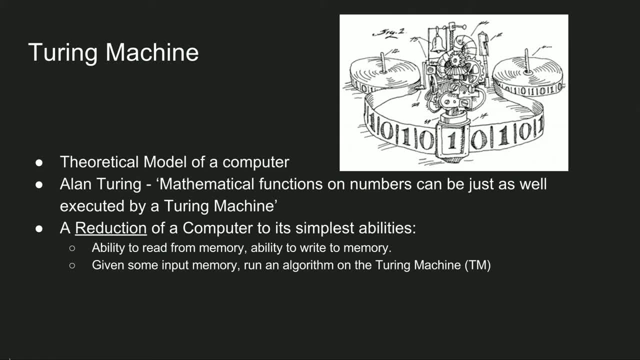 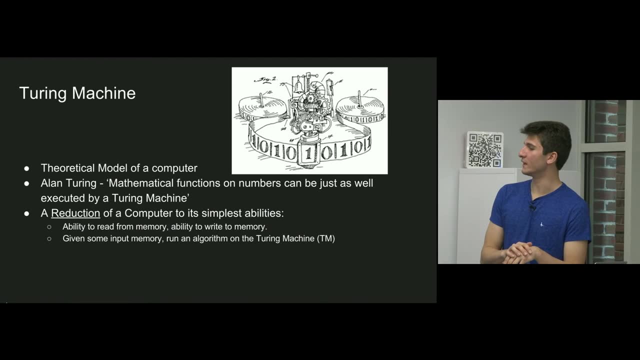 And Alan Turing's saying that mathematical functions on numbers can be just as well computed by a Turing machine. That was basically what was concluded in what's called the Church-Turing thesis, And I like to think of this. It's basically a reduction of a computer to its simplest abilities. 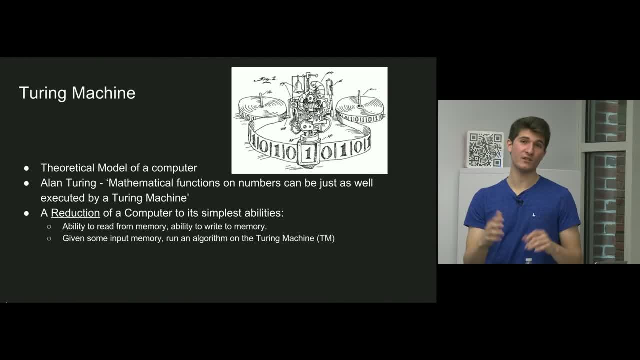 the ability to read from memory, the ability to write from memory, And that's really all you need. You could interpret this Turing machine of just ones and zeros as blocks of eight bits, And then you could have bytes, say, And then you can work in letters, as opposed to just ones and zeros. 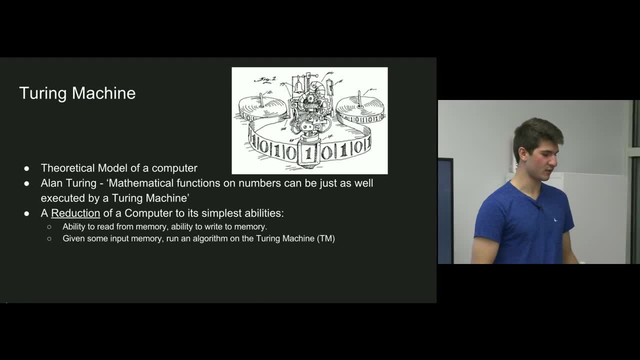 And so far I think reduction is just a concept that comes up a lot in computer science. so it's good to know, And not just in the sense of problems to problems, but also, for example, computers and things that solve those problems. 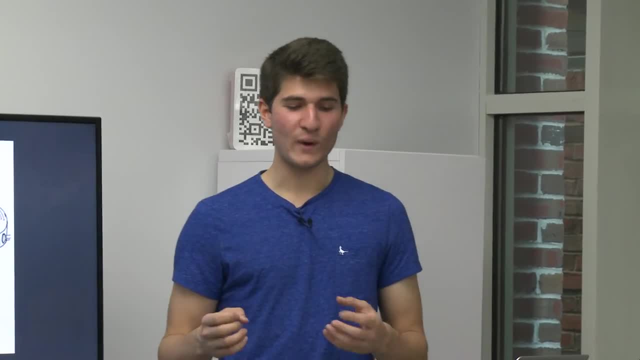 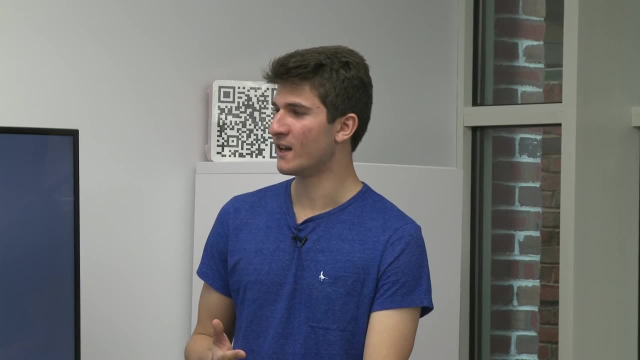 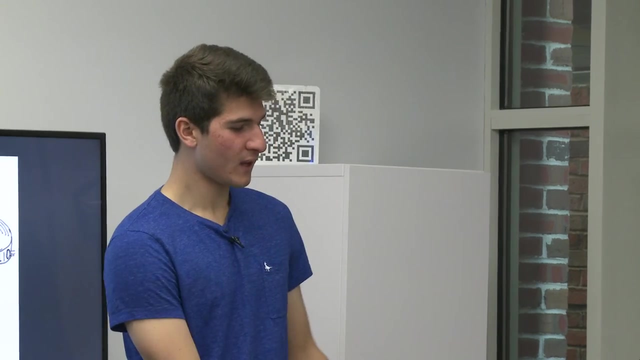 It's worth noting there are also other theoretical ways of thinking about computers. Say, we have quantum computers, which is just another theoretical model of a computer, And that has different ramifications for the P versus NP problem And the problem kind of breaks down in that sense. 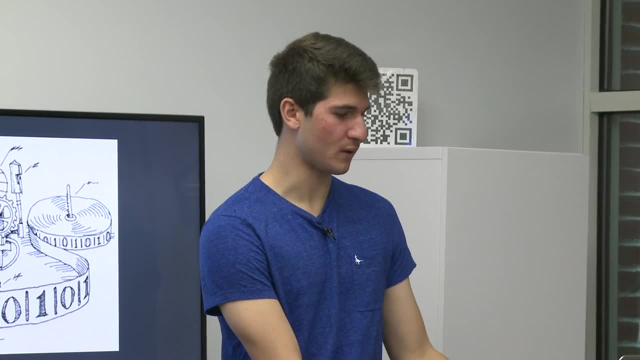 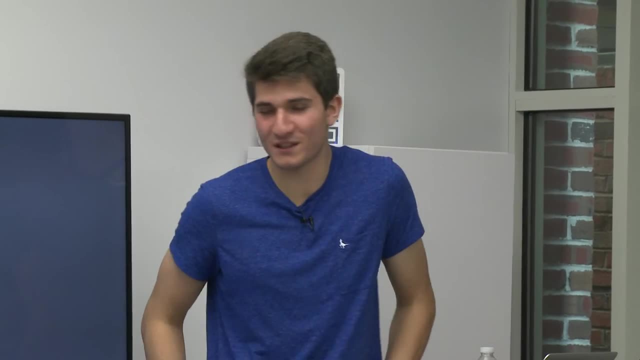 But at least for Turing's notion of computers. this is what we'll talk about. I don't know that the students will let me sit here and talk, But yeah. so what is the resolution to this problem? Is P NP? Is P not NP? 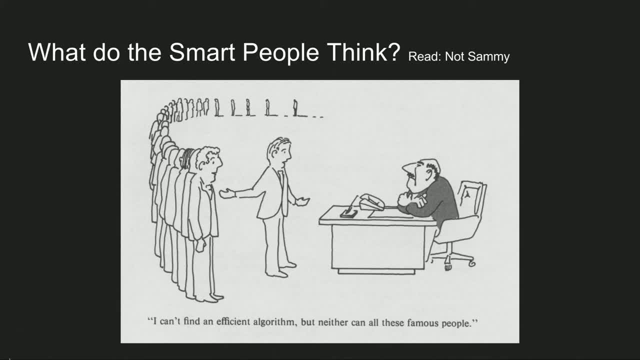 Are these problems? is there a problem that's in NP but definitely not in P, And the answer is pretty unclear. But there's a lot of smart people- not like me, but smarter than me- who think that there's definitely not a solution. 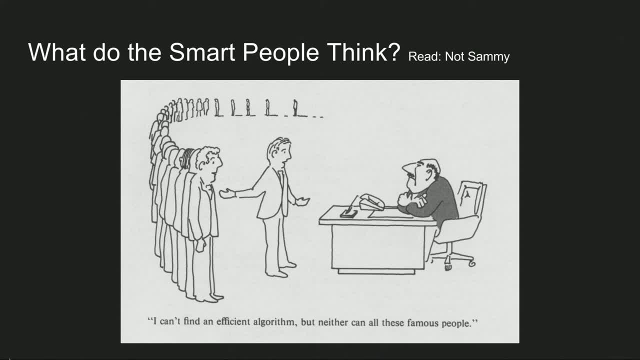 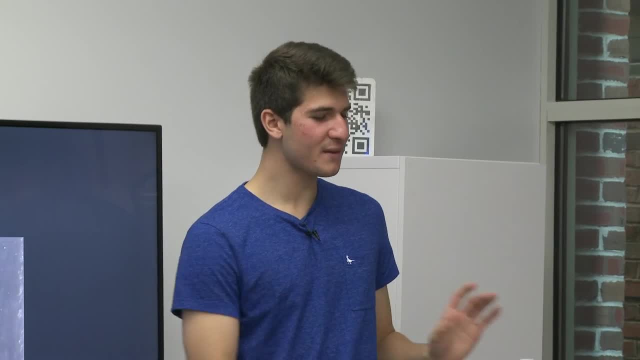 Because people have spent a lot of time thinking about this question and for a lot of these NP-complete problems, efficient algorithms. I think this comic sums that up nicely. So it very much seems like P is not NP. So I hate to break your all hearts, but a lot of people 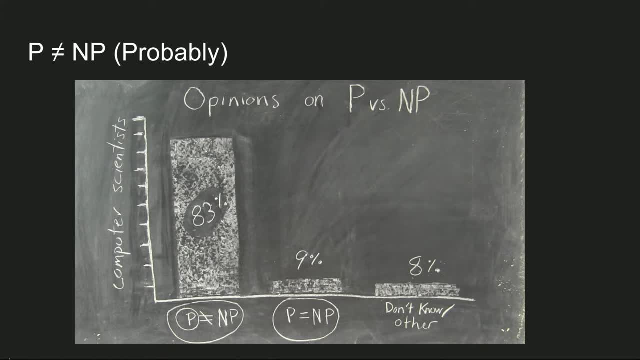 think that P is not NP. There are some people who think P is NP, And then there are the people who have different conceptions of the problem. like well, it's a badly worded problem. Any of the definitions of P and NP are sort of unrelated. 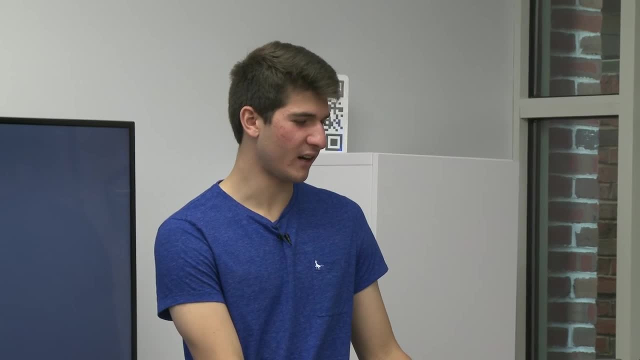 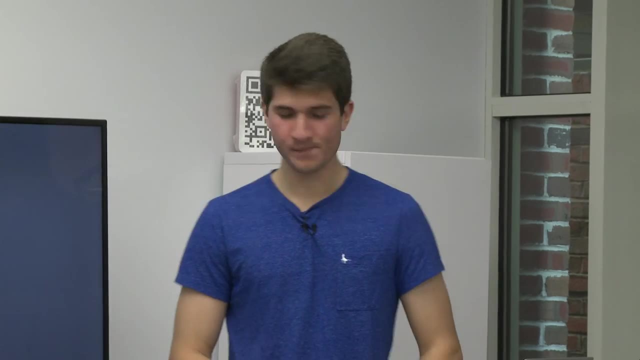 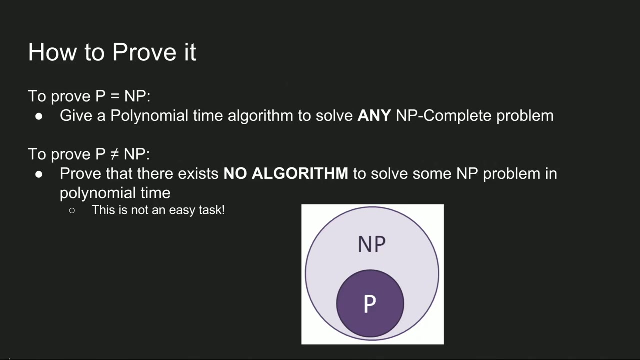 in their definitions. So there's a lot of conceptions, but most computer scientists think it is a well-formed question and that P is not equal to NP. So how would one go about proving this question of the relatedness of algorithm solving problems? 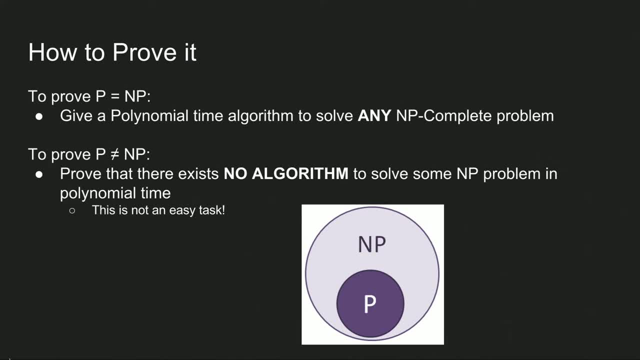 And it turns out it's just not easy, because the way we define these sets is by the existence of algorithms. So to prove P is NP actually is easy- quote unquote- because all you have to do is find one polynomial time algorithm for an NP-complete problem. 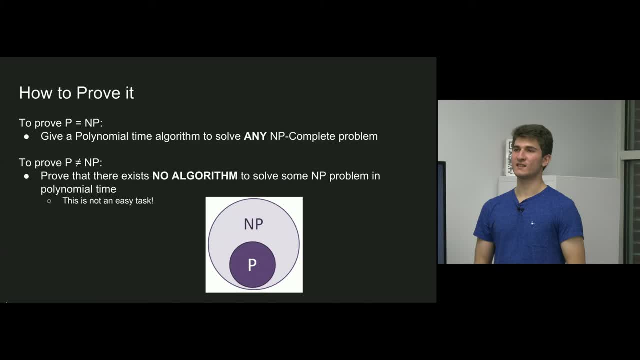 And then immediately the whole class collapses into P. That is because if you had a polynomial time algorithm to solve an NP-complete problem, you could solve all of the other NP-complete problems, because we told you that they're all related by some core completeness. 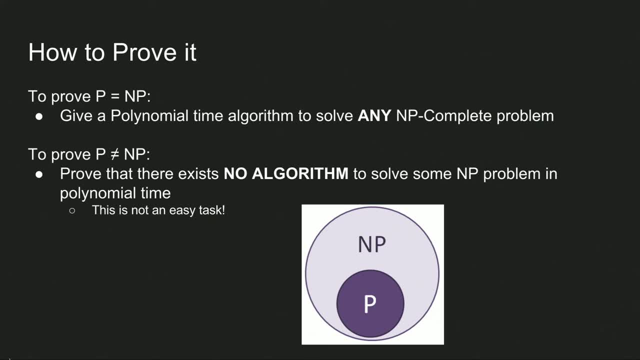 And then to prove P is not equal to NP is much harder, in the sense that you have to prove that an algorithm doesn't exist. And that is actually kind of difficult to solve because in the past we've just invented new algorithms. 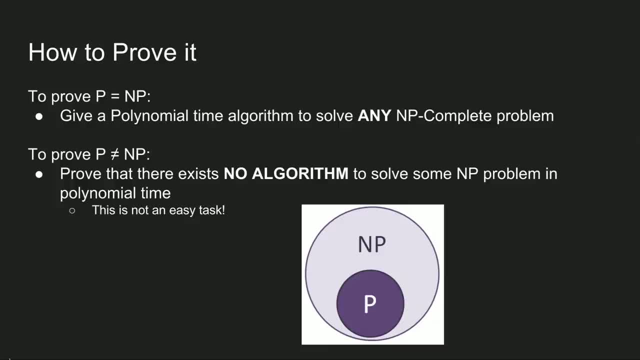 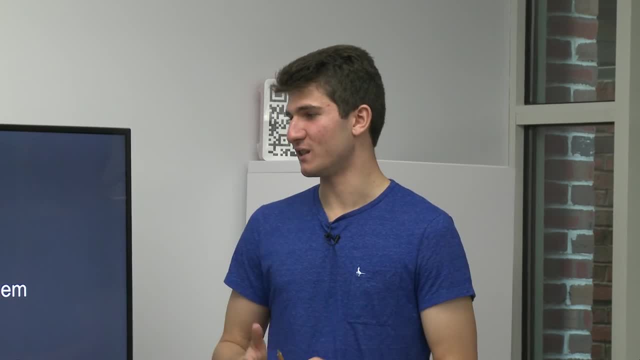 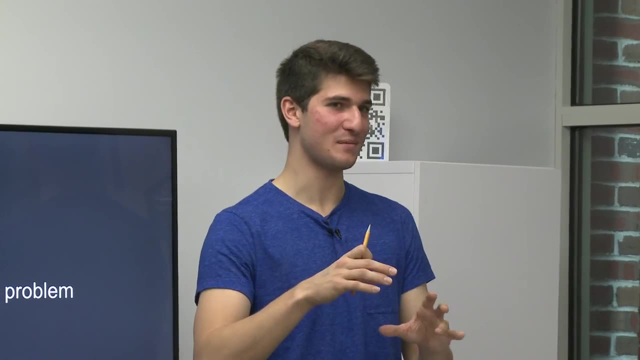 It just took enough time before someone was like: oh well, we can do it this way And we don't have really proof that an algorithm doesn't exist in P. It's only until we just find an algorithm in P that we can be sure that that was in NP and not in P. So that is inherently not. 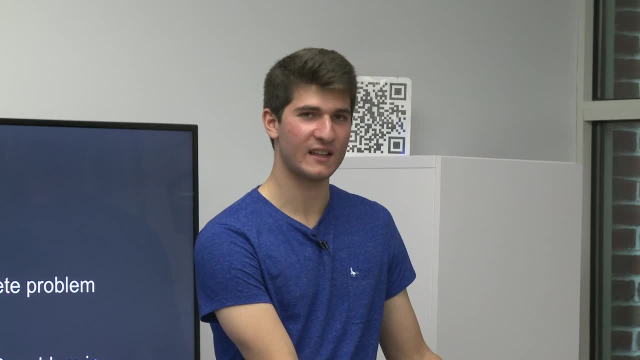 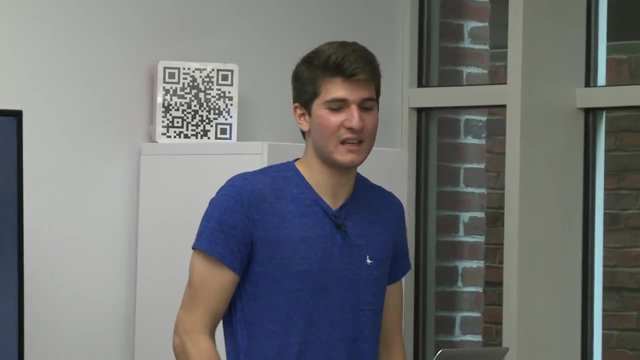 an easy task, Yeah, And I think that's why it makes this problem so fascinating and so frustrating for a lot of smart people. I think one of the most interesting ways to think about this problem is in terms of what if P did equal NP. 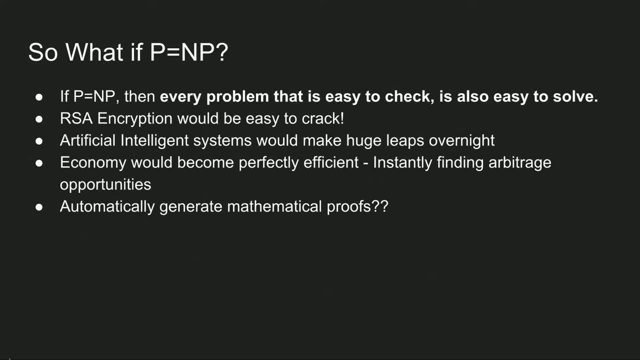 And I think this is sort of like a counter or- excuse me, like a- I don't know what the word is- a contradictive argument where you say: well, what if P did equal NP? And if P did equal NP, then the world would. 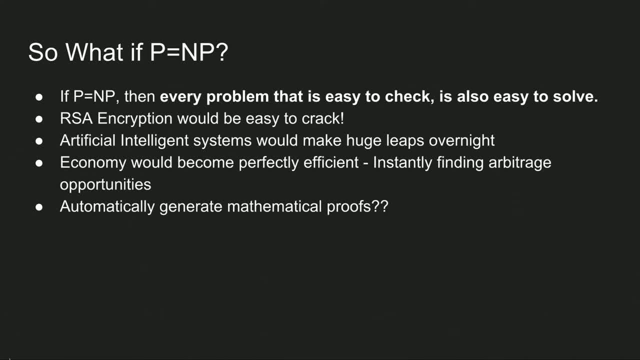 be a lot different. If P was NP, then every problem that would be easy to check would also be easy to solve. What does that mean? Actually, I don't know. I didn't realize this when I first started to research this problem. 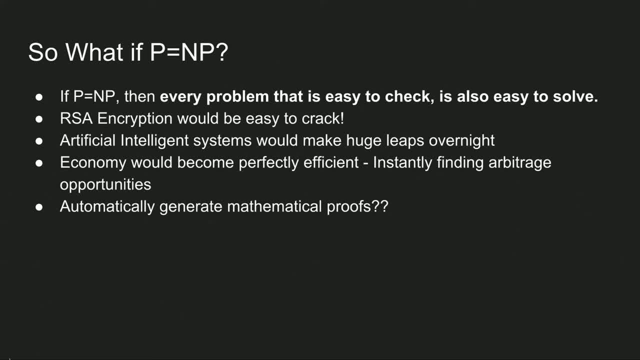 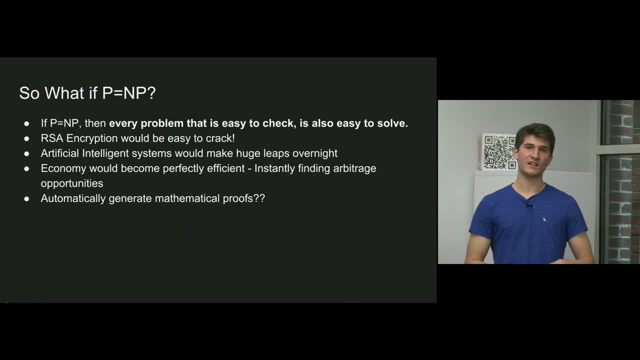 But RSA encryption, which is basically the basis of a lot of our modern encryption, would be very easy to crack because it's based on factoring. It's based on factoring large, large numbers, And if those numbers were easy to factor. 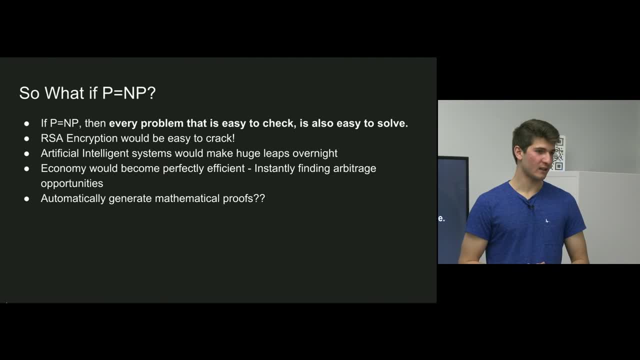 then it would be very easy to basically decrypt a lot of messages that are passed online and things like that. But of course we're relying on the fact that P is not equal to NP and that there is no algorithm that exists currently to do that. 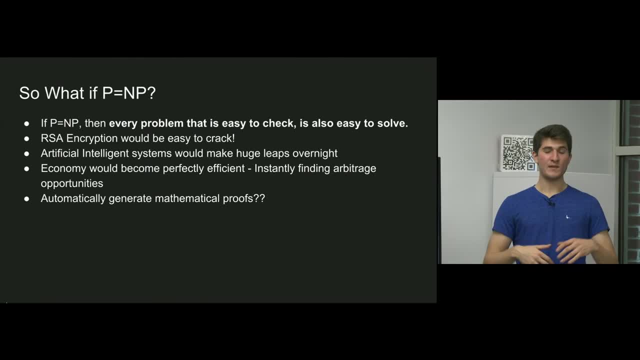 Another ramification would be that artificial intelligence systems would be making huge leaps almost like overnight, because a proof to P equals NP would also tell us something fundamental about solving certain problems that AI people solve. I don't want to go into the details too much there. 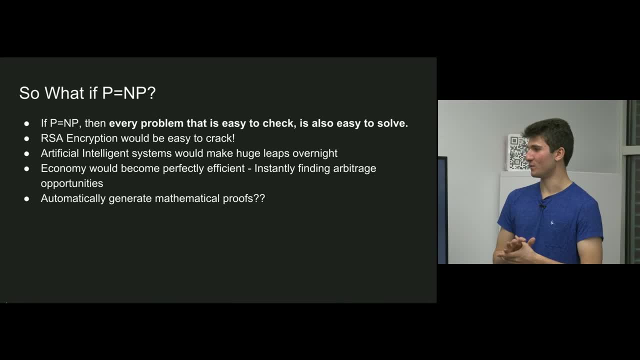 But another ramification, for example, would be that the economy would be perfectly efficient, which means that if there were any arbitrage between two different- well, arbitrage works by taking advantage of the different price discrepancies in a graph, And if those were easy to do, then we'd be able to do that. 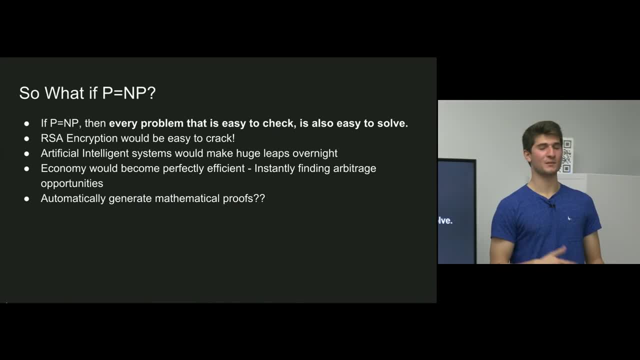 So we'd be able to do that. So we'd be able to do that, So we'd be able to detect, that is, if there were a polynomial time algorithm to detect them, then it would immediately be easy to find these arbitrage opportunities, which 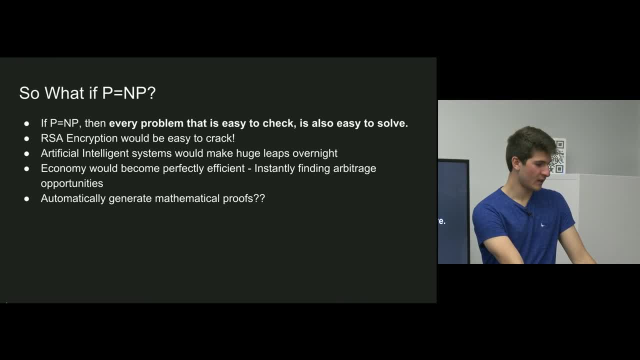 is sort of a very bad thing. And then another thing would be: a lot of people say that proving things or mathematical proofs is such an NP problem, Because, while it's easy to check if a proof is correct, you just follow the logic. 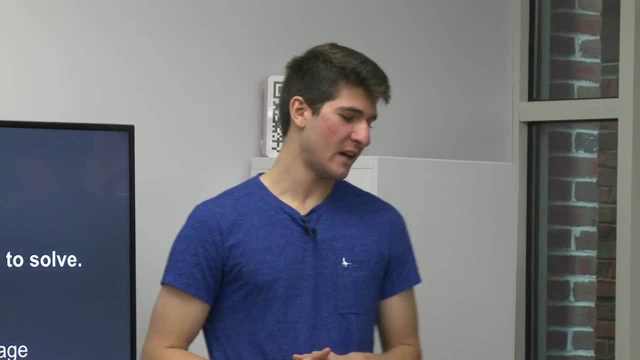 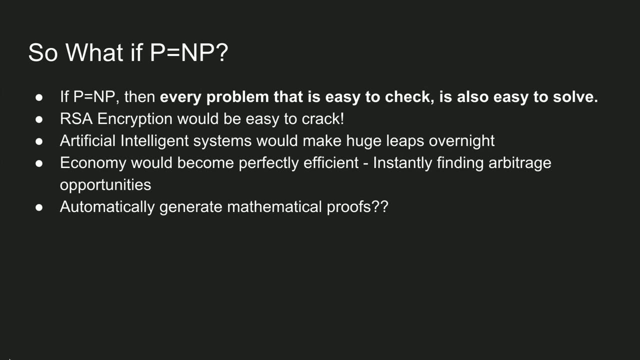 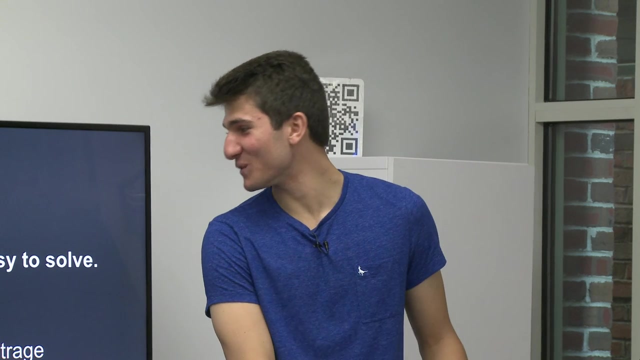 It's much harder and it's a creative task to actually actually create a proof, And so we might be able to write computers, write programs that make mathematical proofs if P did equal NP, which would just be crazy And that would just make the whole world explode. 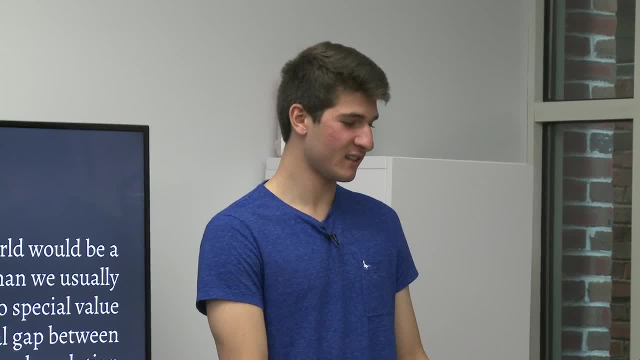 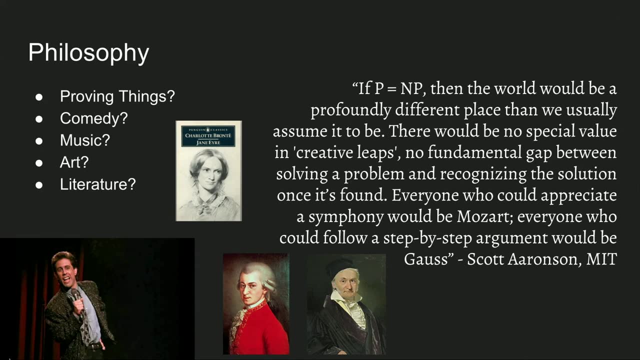 The world would be fundamentally different than the way we currently think it is. And a little more philosophy here, which is one of the fun things I like to think about, is proving things Well, we just talked about. it is sort of like an NP problem. 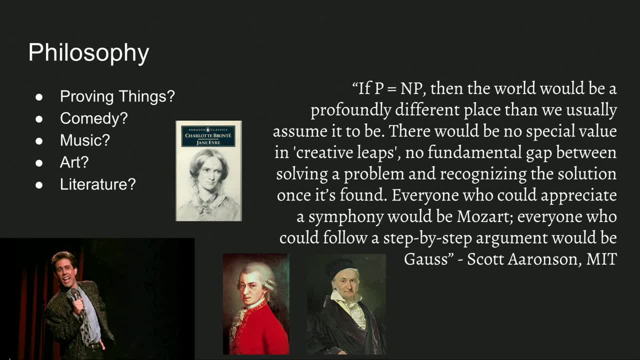 because you can just follow the logic and it's easy to check. Is comedy like an NP problem? I mean, if I tell a joke and you laugh at it, then it's really easy to check that. that was like a funny joke. 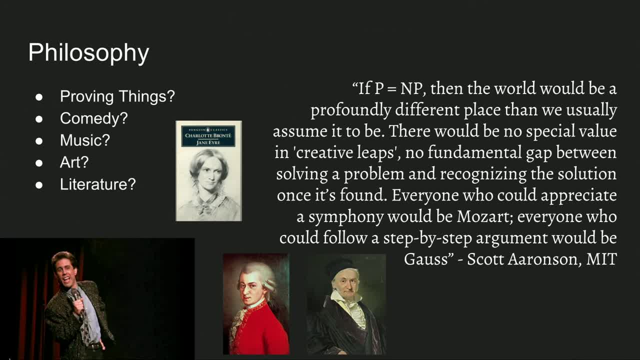 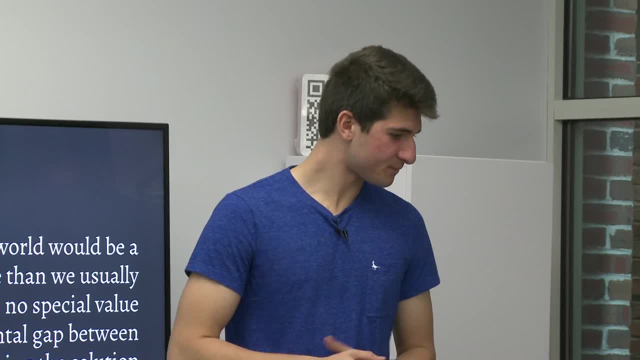 Much harder task to write a funny joke. I know because I do stand up and enough people have sat in silence at my jokes. I know it's a very hard thing to do. Music- appreciation of music. Is it an easy thing to check? 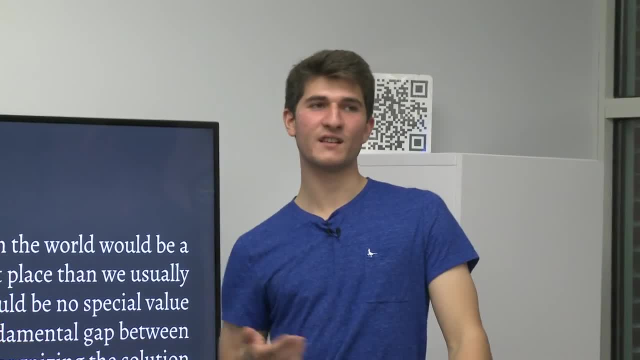 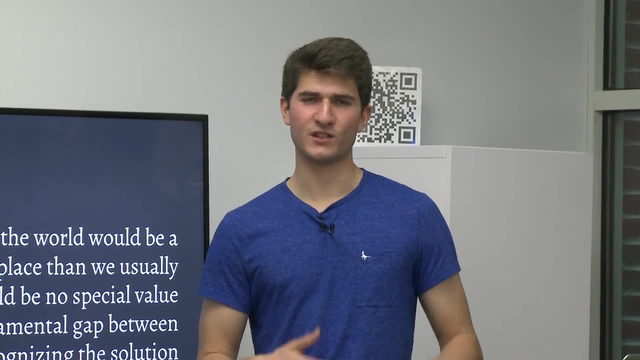 Well, yeah, I mean, if you just listen to something, you can kind of intuitively tell that that is a nice sound, But it is actually much more difficult to create music, create good music, And that is. these are all sort of philosophical arguments. 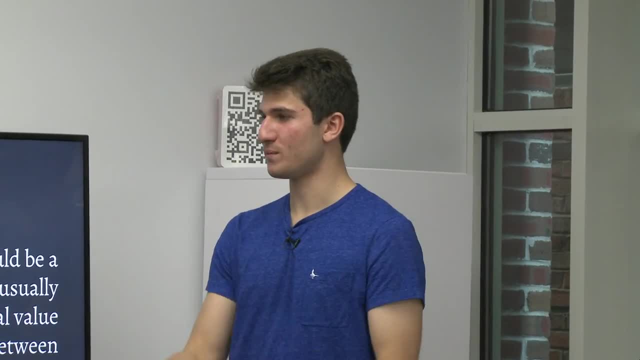 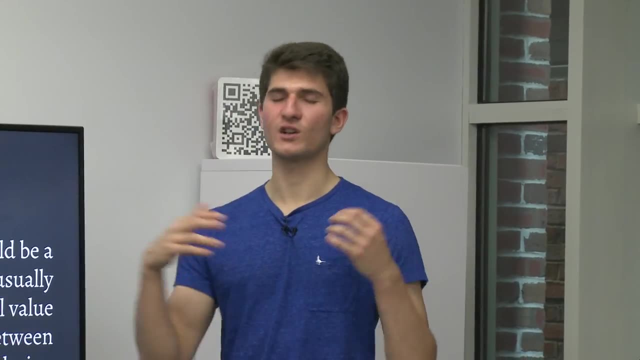 These aren't really the actual definitions of P versus NP that we're exploring, have a much more well-defined relationship to Turing machines and what are called languages, But when we think very highly of something, at a very high level, the ramifications are sort of endless. 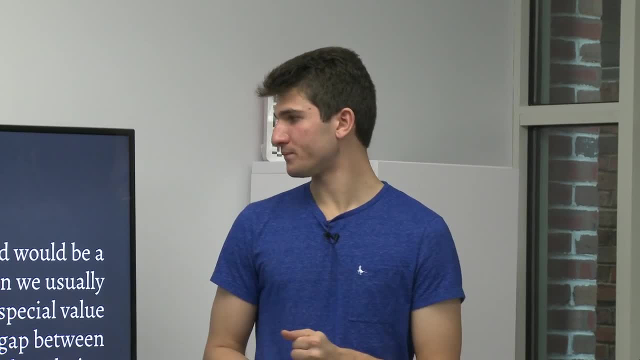 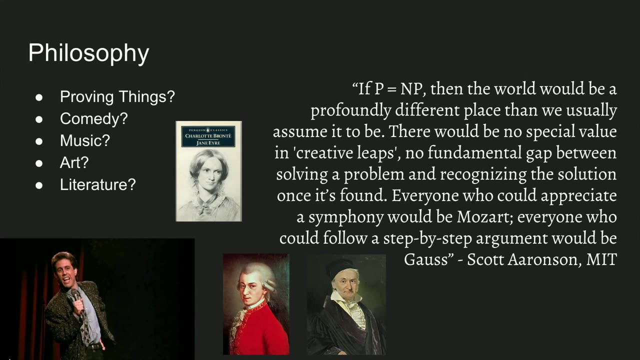 for any sort of creative pursuit, And Scott Aronson of MIT once said that if P equal to NP in the world be a profoundly different place than we normally assume it to be, there would be no special value in creative leaps. There would be no fundamental gap between solving a problem. 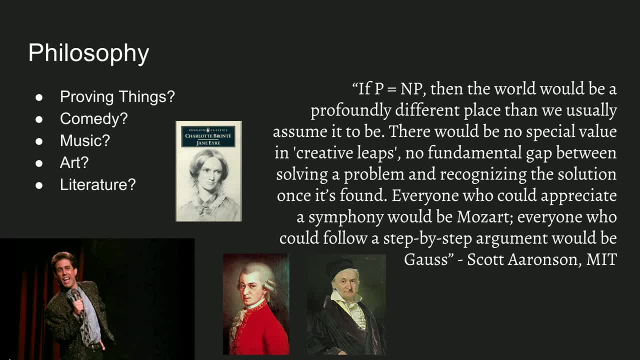 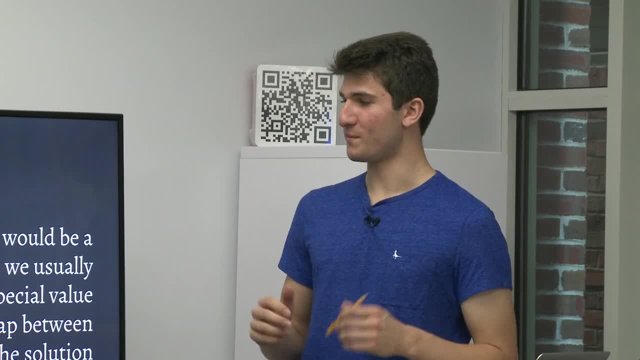 and recognizing the solution once it's found. Everyone who could appreciate a symphony would be Mozart, and everyone who could follow a step-by-step argument would be Gauss. I think that sort of tells you something about the crazy, crazy ramifications of a proof that P did equal to NP. 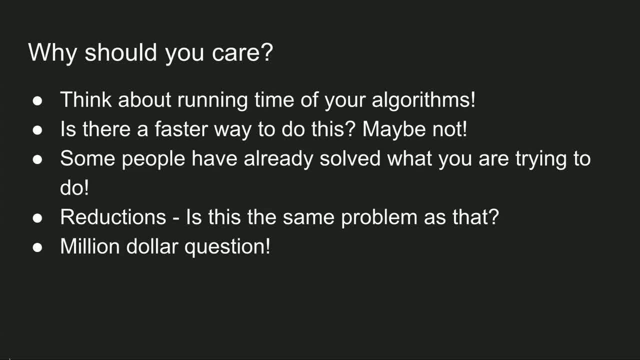 Yeah, so why should you care? I mean, hopefully you're sitting here and being like: well, that's great, but I have a final project to do And this doesn't really help at all. I don't think many of you are going to be doing theoretical proofs or anything. 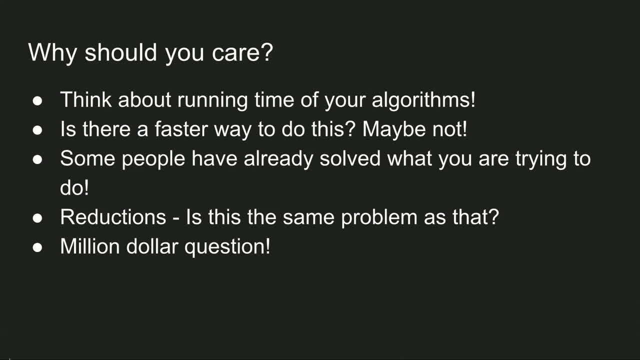 like that, or talking about theory, Although I think you should. I mean, we talk in CS50 about running time of different algorithms, and that is very relevant Because There could be a faster way to do the problems that you're thinking about. 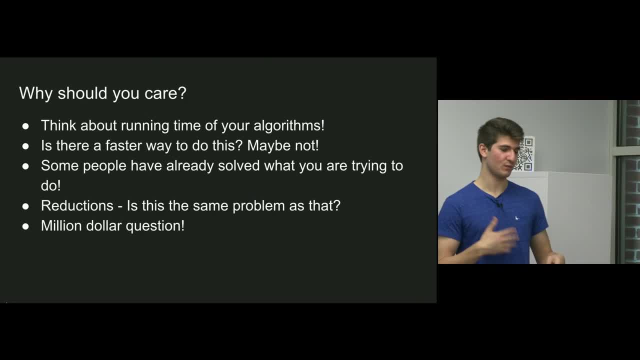 You just don't know it yet. And that's why theoretical computer science has researched the fastest way to do certain things And that's why reductions have shown us- reductions from NP, complete problems have shown us- that if a problem existed, this problem a problem. 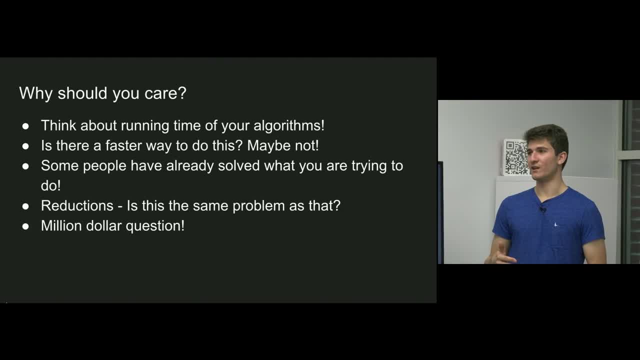 that you're trying to solve might actually have already been solved. Or another thing is that, well, if you assume P doesn't equal to NP, something you're trying to do might not be there. It might be that easy to do, And if that wasn't motivation again for why you should care, 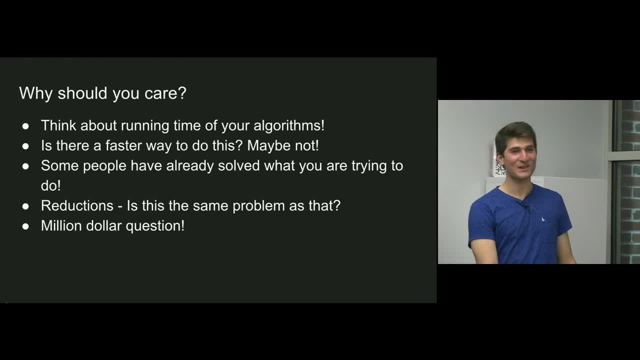 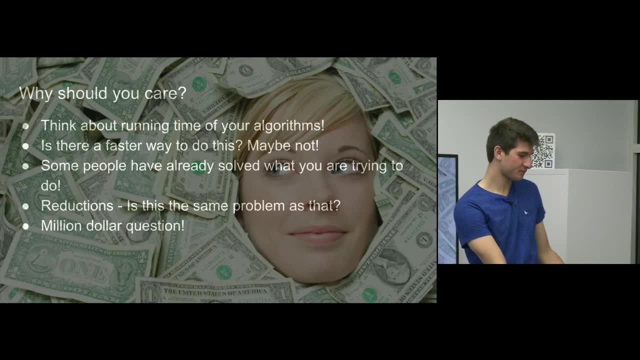 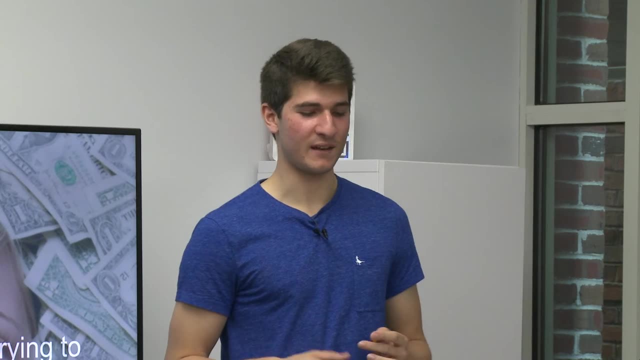 well, it's a million dollar question, right? And there's nothing that computer scientists like more than computers, except for money, right? So I think that should be motivation enough for you to be interested in the P versus NP problem. It is something that is really interesting to me. 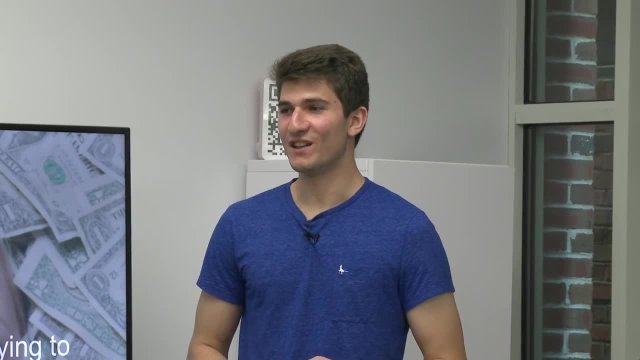 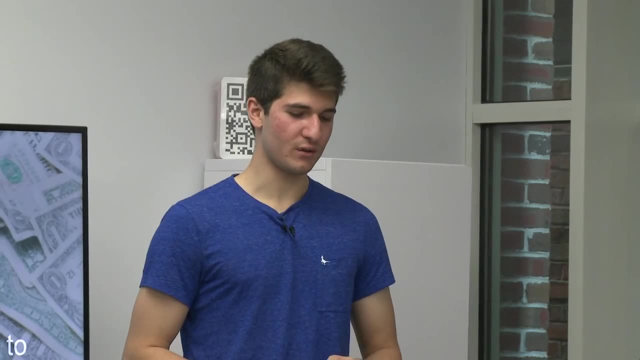 I know I took you through the weeds a little bit with the actual reductions, But I hope that was interesting. And that's really what computer scientists do when they think about these types of problems, is reduce problems to another and sort of relate these algorithms. 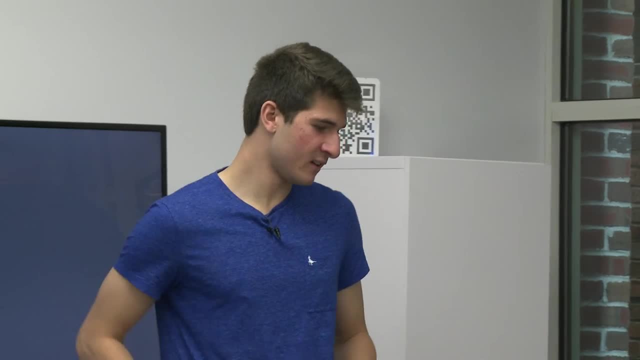 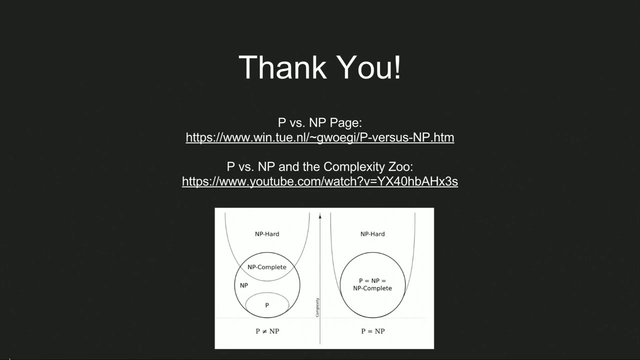 And so I think that's about all I have, But I hope you enjoyed. Here's some links. just the P versus NP page. It's sort of like a collection of the status and history of the problem And this is just a video I really like that explains all these things very. 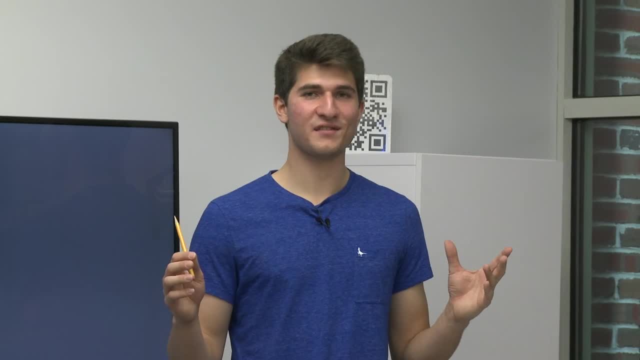 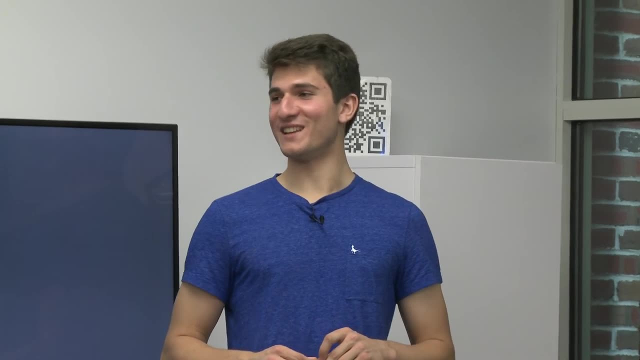 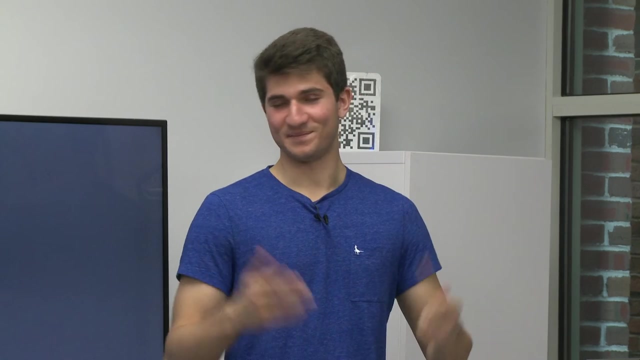 well, So that's all I have. I hope that was enjoyable for you And for everyone out there enjoying it on YouTube. I guess I hope you could take something away from this. And yeah, I mean P versus NP. it's pretty cool.